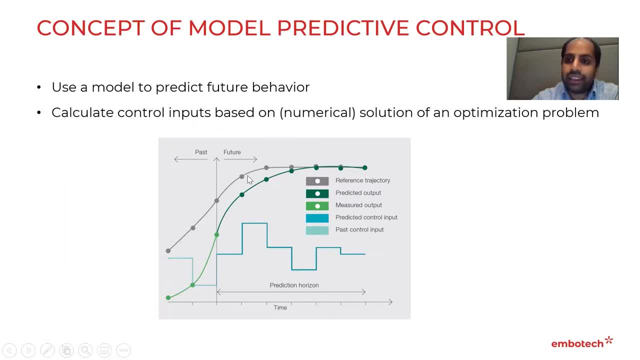 predicted outputs and the reference values, and you set this task up as an optimization problem and then you actually solve it and by that you get the best possible control inputs, for example, as I said, to be as close as possible with the predict outputs to the reference trajectory. 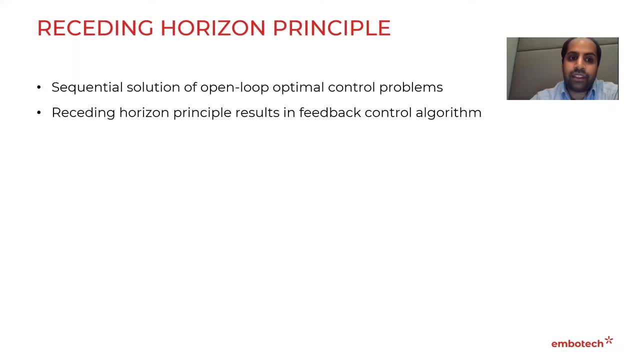 And what is done on top of that is you solve this open loop optimal control problem sequentially. and this is actually called receding horizon principle, because what you actually do- and that's what we see here- you plan for a certain horizon, but you only apply the first control action, and that's what you do, and you discard your entire rest of planning. 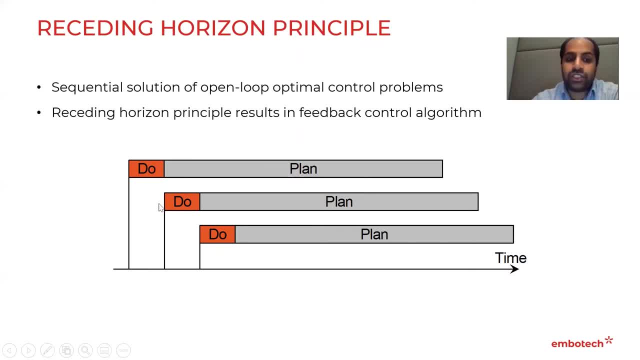 and then- and now here comes the receding horizon- because you shift this horizon, because now you have evolved in time and you plan and again, and you actually apply again your first actions and you discard the planning again, and then you do it over and over again, and because 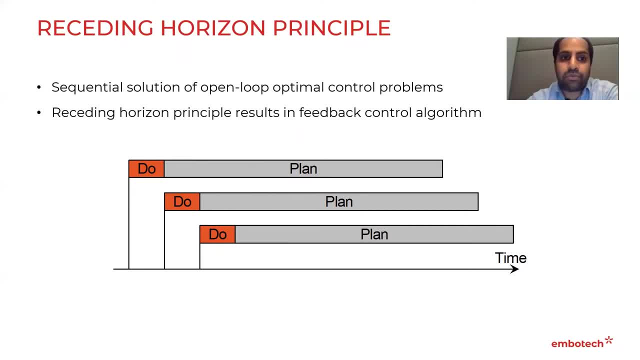 you shift this horizon- it's called actually receding horizon principle- and if you do that- actually, because you always take into account your new situation- so this might be your system states, but also your disturbance values- you actually have a feedback control algorithm and every time when you do this planning, this is an open loop, optimal control problem, because 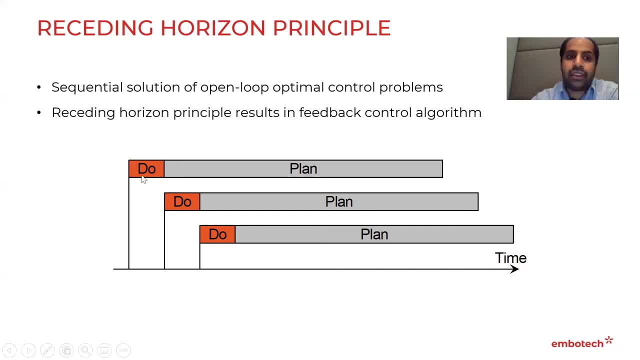 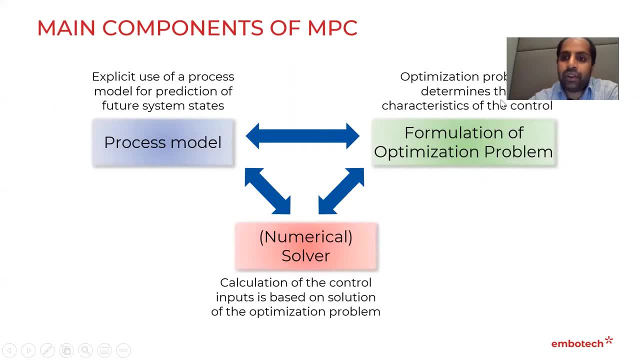 you plan based on what you know of the future and you solve it over and over again. So what are the main components of model predictive control when you design and control algorithm that you need to take care of? So you have the process model and you need to have an explicit process model for prediction of future system states and, as I said, 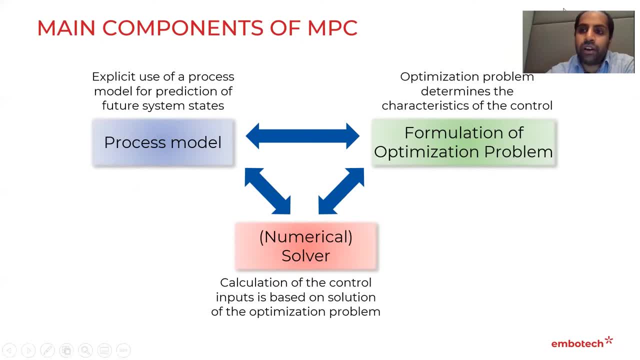 this is a mathematical model, so it could be a state space model or an ordinary differential equation system, And so you, as a user, you have to actually have this process model that describes your system. then, at the same time, you need to have a formulation of your optimization problem. 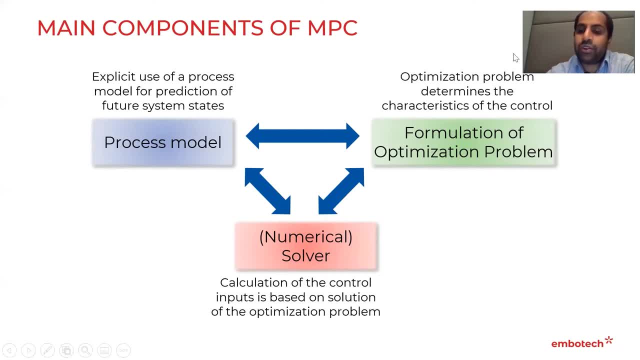 and because the optimization problem at the end determines your characteristics of the control, and so you need to think about other requirements for your control algorithm and, based on that, you need to appropriately formulate this optimization problem. So now we have the process model and the formulation of the optimization problem and, as I said, typically what is done. 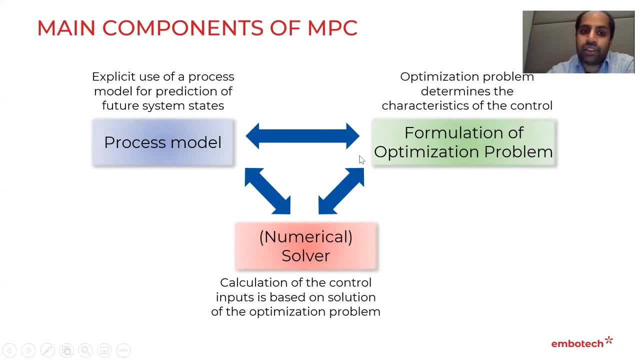 during runtime of the process, you solve this optimization problem, and so you need some numerical solution algorithms- which is called solver- that calculate the control inputs based on the solution of the optimization problem, and that's these three components are the the main three things you need to think of when you actually design an MPC algorithm and, as you can, 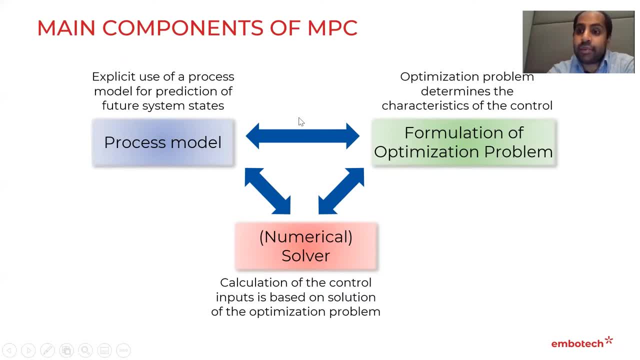 see, depending on the system you want to control, you might think of different ways to actually having the solver or the process model or the formulation of the optimization problem. so the biggest challenge is actually real-time feasibility, because you typically have very small sampling times and you need to be sure that you can actually solve. 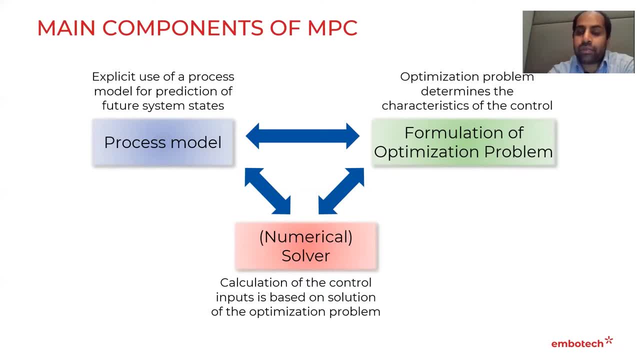 your optimization problem in this time frame and if you would have a very complex process model, of course the optimization problem would also take quite a lot of time. so you need to make sure that for appropriate control all of these three parts, that they fit and that you actually are able to deal with it. on the other side, if you have a very simple model, 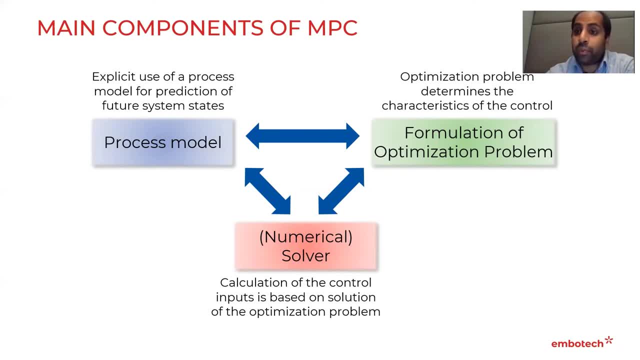 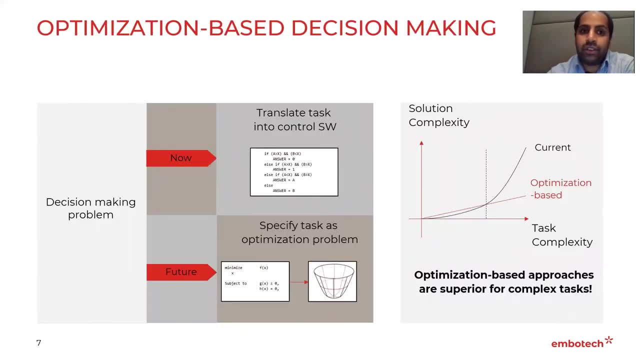 it might be actually too simple, because you not describe appropriately what your system is actually doing and what is actually the reason that we do this optimization based and let's call it in general, decision making, and so we have this decision making problem and what you would do and what is the standard in the industry. still, 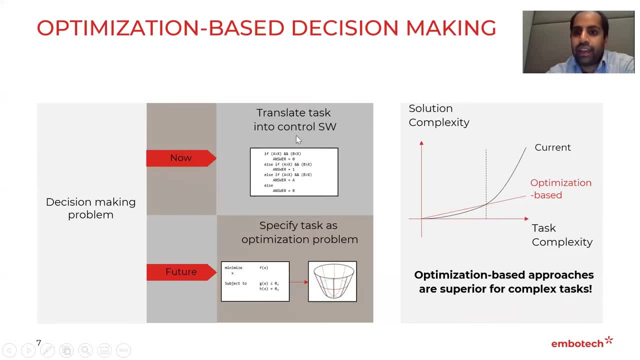 is that you translate your task into some control software and in some cases this might be that you have a lot of, if else, admins and, depending on what happens, you actually change. it might be also look up table based controller where, depending on operating point, you also change. 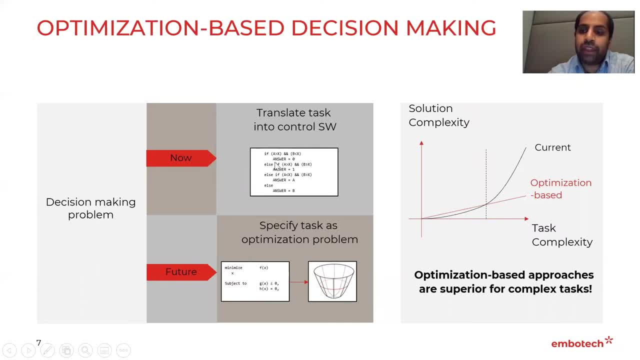 your parameters, but it is very, very dependent on different states and then your software needs to take into account this state dependent behavior and but what we think is going to be the future is to specify actually your tasks, your engineering tasks, where you want to solve your decision-making. 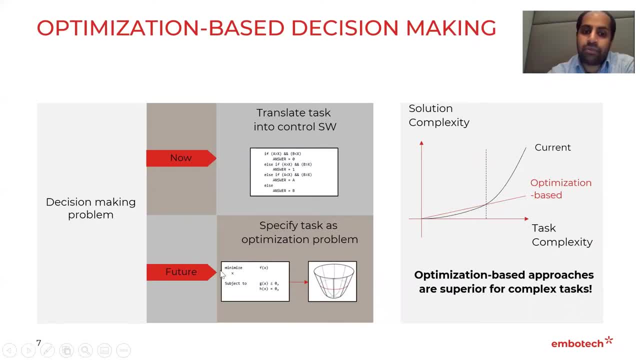 problem that is specified as an optimization problem and then solve it actually. what is the big benefit? like looking on a very high level on it, and if you have a task that is quite easy, then you are actually better with dealing in the fashion to translate the task into a control software. but if the task gets very complex, 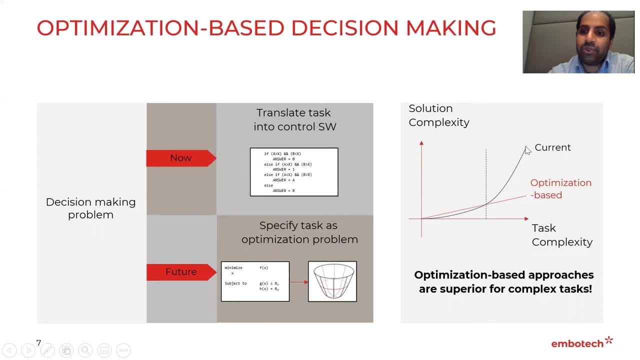 then actually, your solution complexity will exponentially increase, and if you have put it as an optimization-based task, it will just literally increase. so it's, if you have these very complex problems, it's much easier to solve them with optimization based methods compared to the ones that are currently available. and so let's look at the two main applications, i would say, of 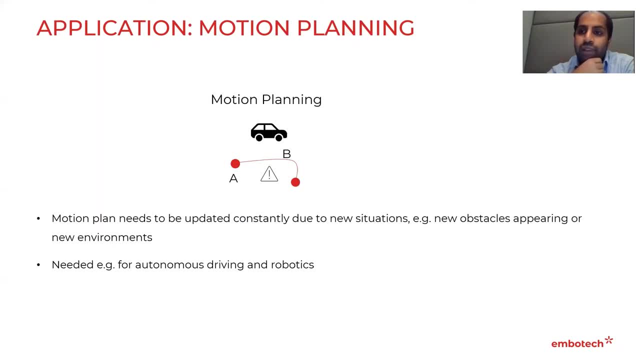 model, predictive control. so the first one is actually motion planning. so you have, um, let's say, for example, autonomous driving, where you have a car that you want to drive autonomously, or you have a robot that should be operated autonomously and the task is to go from a to b and you have 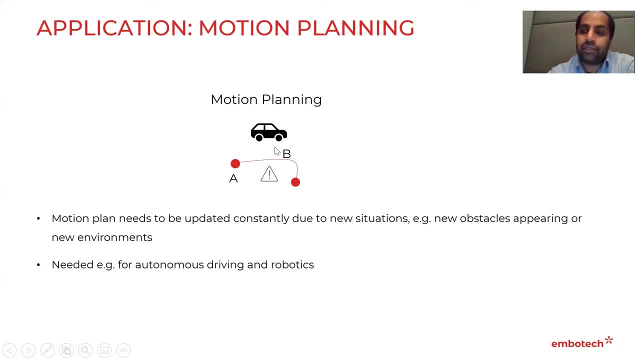 obstacles in the way and you need to find a motion plan. this avoids, for example, the obstacles. in some applications you have on top the requirement that you want to be as fast as possible. other than others, you might want to go there with low excitations so that it is comfortable. 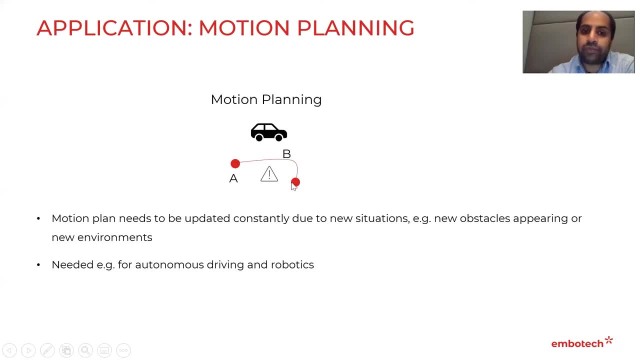 and you need to find the best way to go from a to b and at the same time you always need to take into account that the obstacles might change actually during runtime. so if you think of a car which is driving on a highway, then you always have different situations. 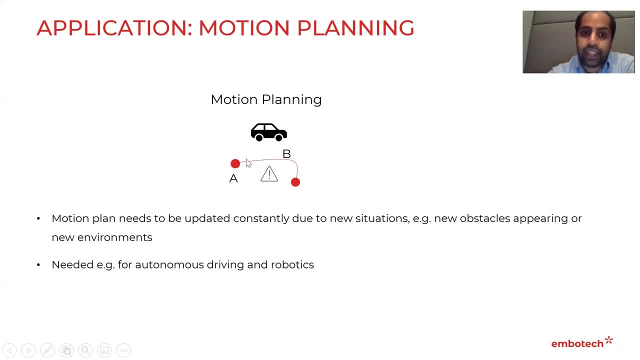 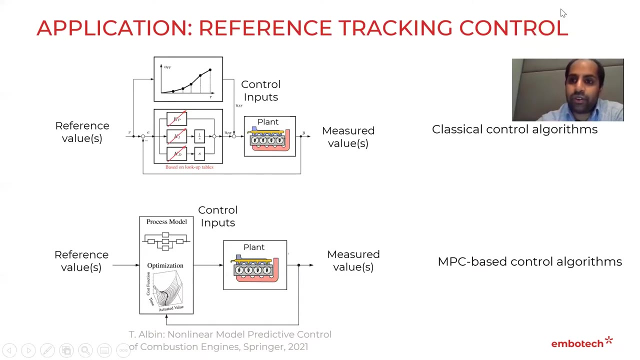 so you need to constantly update this motion plan, and here also, mpc is a is a superior method to actually deal with these kinds of problems. the another one- so that's the very classic one- is reference tracking control problems, and so what you have is you have a reference value which should be set, point tracked, and 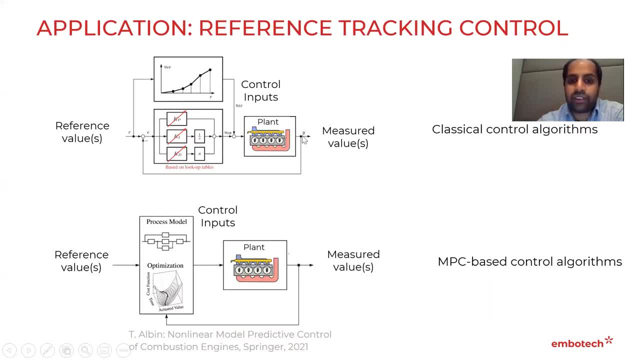 you have some plant that is to be controlled and you measure actually your values and that are your outputs of the plant. you feed them back compared to the reference values and classically you would do that with um, a two degree of freedom controller, so you have some feed forward control. 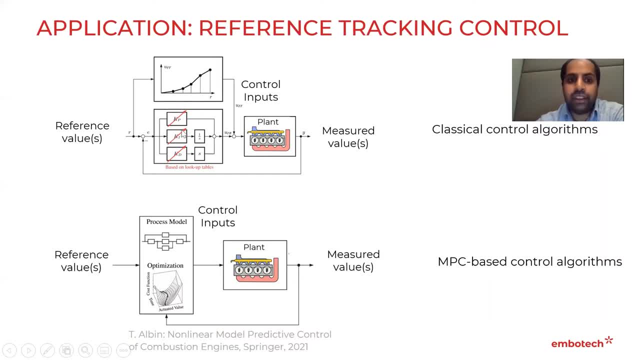 action and you have some feedback action, for example, a prd controller, and if you have a non-linear system, then you that you want to control, then you typically one way to deal with the non-linearity is actually to use lookup tables and then your parameters- kpki, kd- they get. 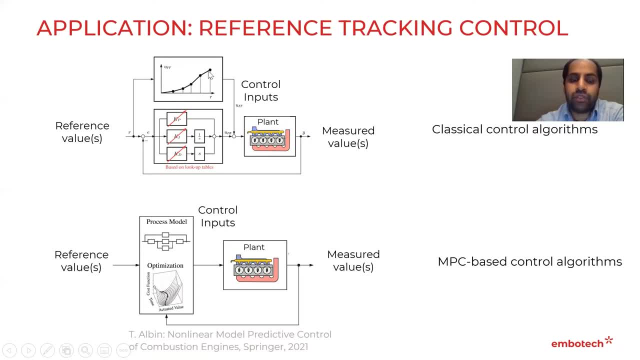 operating point appointment, and the same holds true for the feed forward control. so you have operating or, for example, reference point added from the non-linearity луч, and then, when you haven't used ratchet and blueprint control yet, you need generally kind of republican easy pen run. 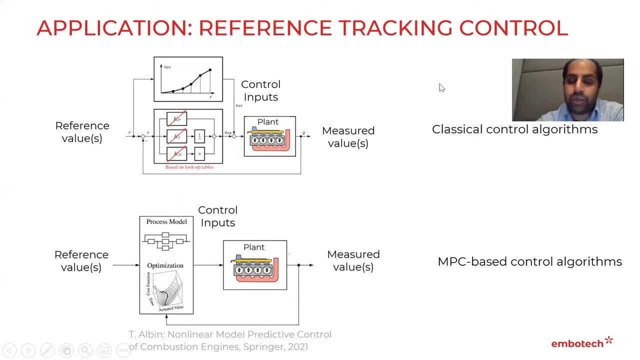 point-dependent feed-forward actions. If you now substitute this by an MPC-based controller, then you don't have the division between feed-forward and feed-back anymore, but you replace it actually by the MPC, and the MPC contains the process model and then the optimization algorithm and this calculates. 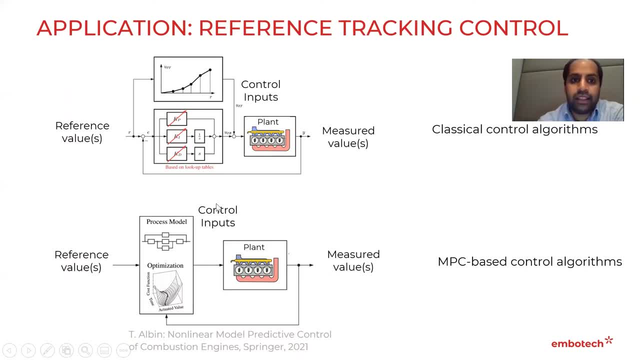 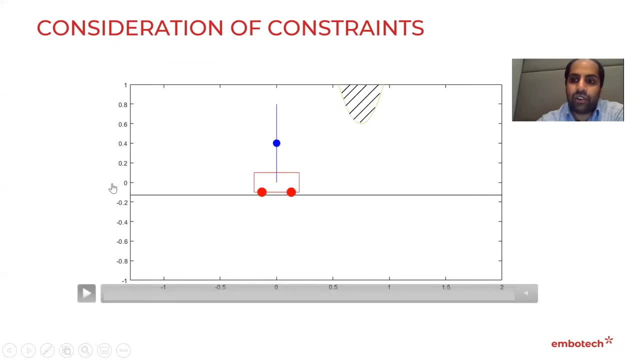 actually your control inputs. So to show you just that, the MPC-based approaches, that they are capable of solving more complex problems than you would be able to do with the standard approaches. I have one example. So a classical control example is the inverted pendulum, where you have a card and you have 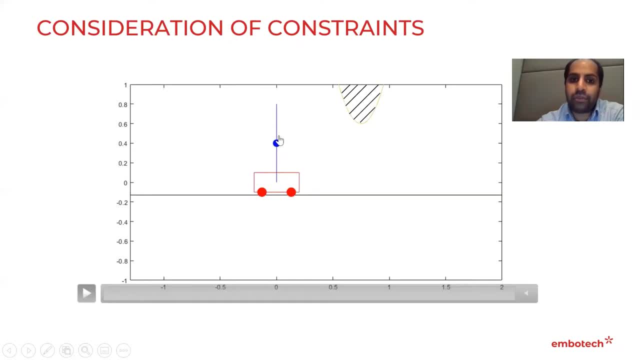 a pole on the card and you try to balance this on the upright position, which is unstable. And now what you can do with MPC. So we have this position A, B. We assume that we have some obstacles which are shown by this black marks, and we want: 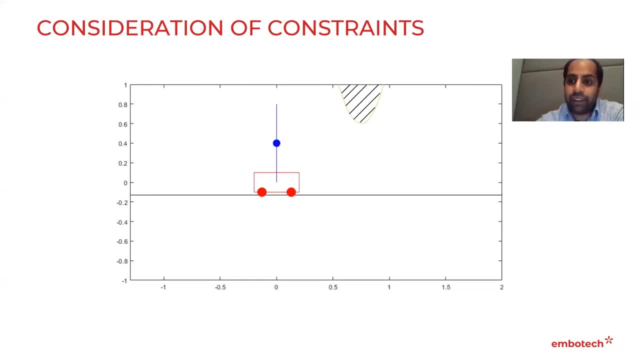 to go to B and we want to go from A to B actually in a time-optimal manner, Then I can show you what the MPC-based solution actually makes. So it takes into account that there is this obstacle and in order to go from A to B, 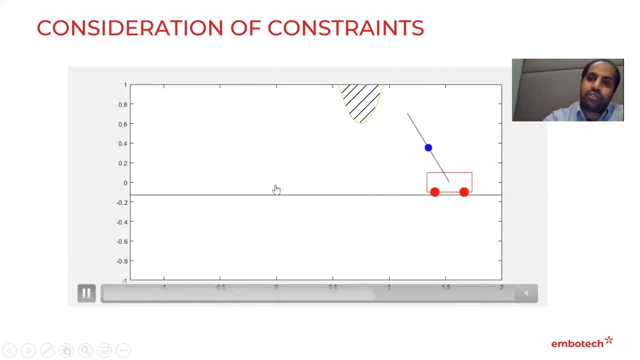 you actually at the very beginning, which might be counter-intuitive- you have to drive backwards and you see it systematically takes these obstacles into account And it just doesn't. goes exactly to the lowest point and then goes from there to the point B and 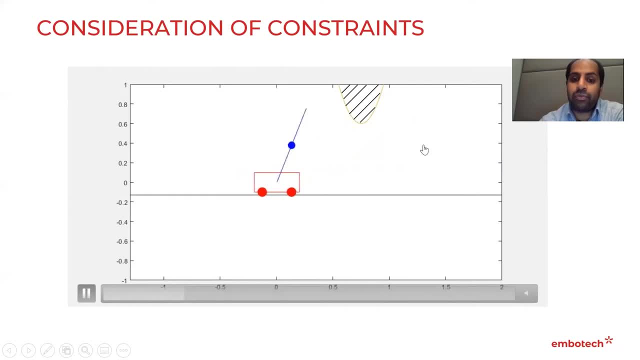 so we are really optimal in how we go from A to B, and this is, of course, very complex. if you want to solve this with an PRD based controller and if you assume, like this obstacle, you would just increase it in an MPC based fashion. you just increase the parameter of the obstacle and then you have to algorithm. 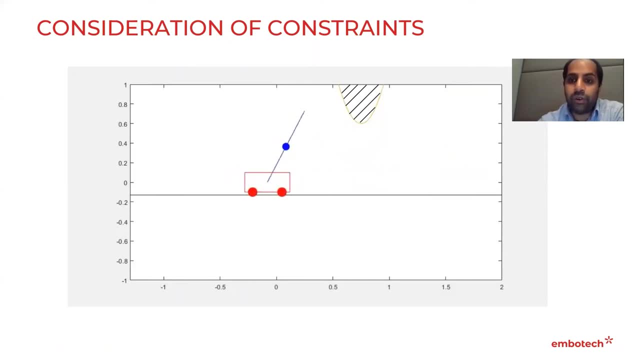 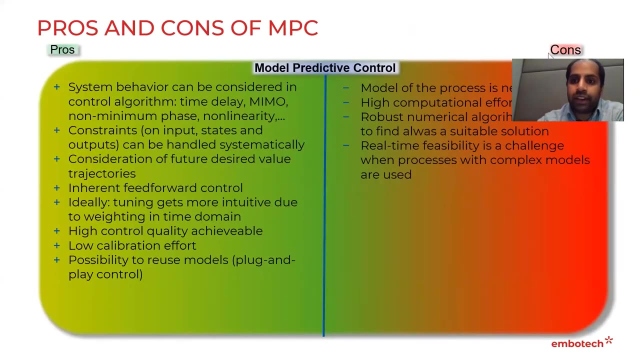 in the PRD based setting, you might to retune your whole algorithm again. so let's look a little more in detail. what are the advantages and disadvantages of model predictive control? actually, because we take into account the model and then do this optimization, we are actually quite 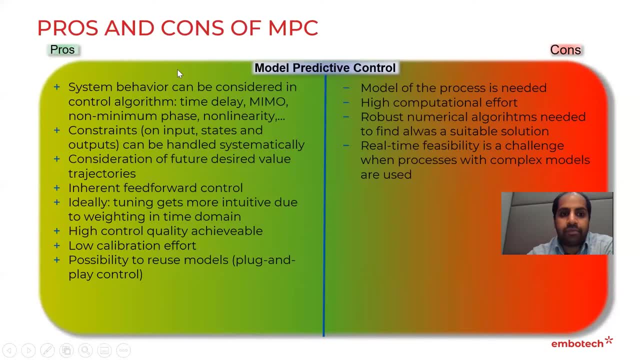 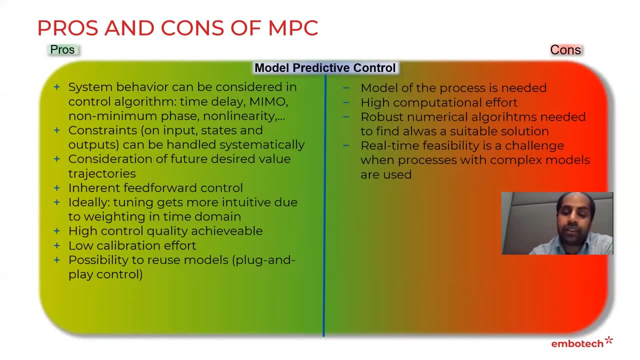 and a lot of other features, because you actually model them and as long as you can model them and you're able to optimize for them, you can take into account of them in a very systematic way. and then, as we have the optimization problems, we are also able to include constraints, and these can be constraints. 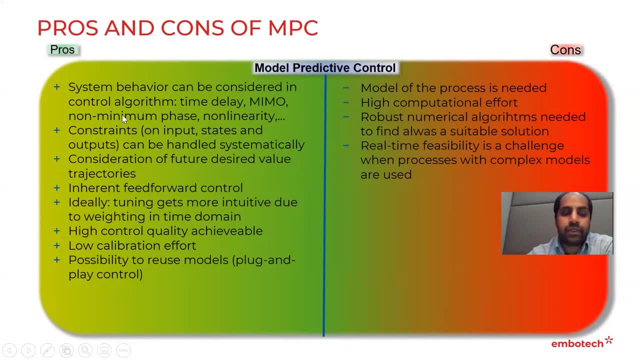 on the inputs, on the states, and on the outputs and MPC. that's like the biggest advantage compared to other classical algorithms that you can actually systematically take these constraints into account. If you take the system behavior, for example, depending on the system maybe there are different control areas which take care of them, for example, your time. 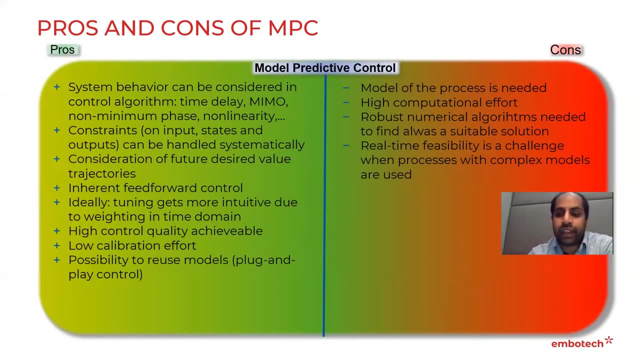 delay, you might take a Smith predictor and so on. so there is different ways to deal with it. but with MPC you are very systematically able to do it. you don't need to have several features and you can at the same time consider the constraints. but you can do on top is you can consider future desired values. so if 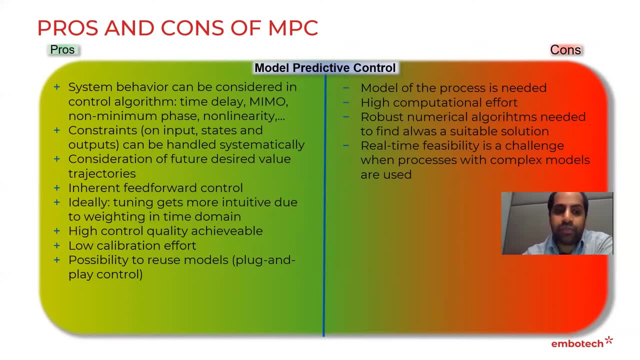 you know and that you future. there are some disturbance values upcoming or, as in the case of the motion planning, there's an obstacle in the future. you can easily include or consider these desired values and, as said, like classical control, use feed forward plus feedback. here the feed forward. 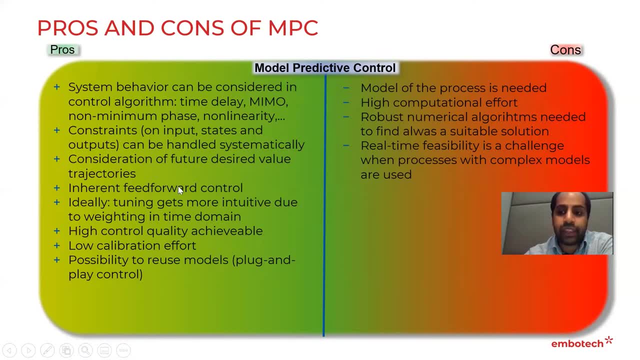 control is inherently included and because- going to next was point, because we do set this as an optimization problem- we have the tuning in the time domain, which is often more intuitive than tuning the control algorithm in the frequency domain, and because we are able to take the non-linearity into account, the time delays and so on, we actually can have a very high control. 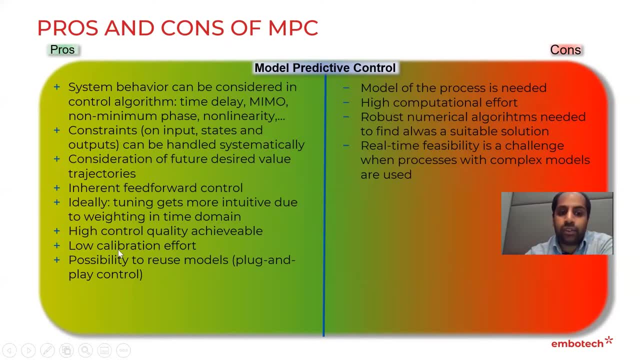 quality and because we do take into account directed nonlinear system behavior, for example. so we have also low calibration effort. just think of it. if you have a very nonlinear system and you need to tune for it at different operating points, then this is much more tedious as if you just insert your nonlinear system. 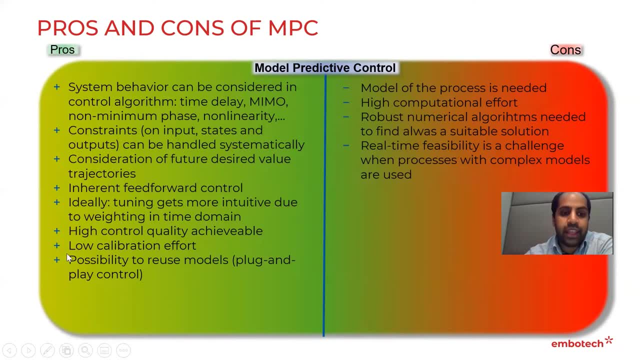 behavior and directly use it. and the last point is the possibility to do to you reuse models. so let's take the example of motion planning. so if you have a vehicle dynamics model, then even if you change your vehicle uh certain parameters, for example tire coefficients, you can still reuse the entire model without the need to come up with a completely new control. 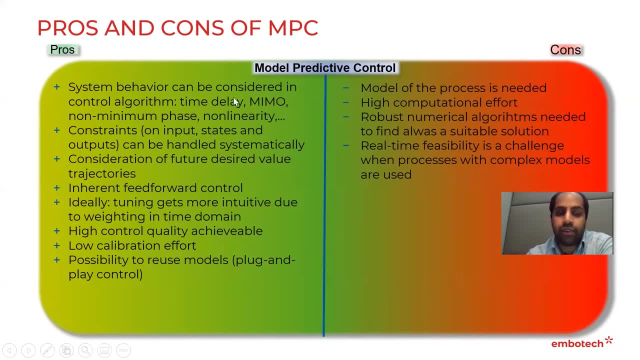 algorithm and this is sometimes the case. assume you have one system and which has no time delay, but then you include a new actuator which has some time delay. it might be that you need to enshrine entirely, change your control algorithm. but with npc we just include the time delay and 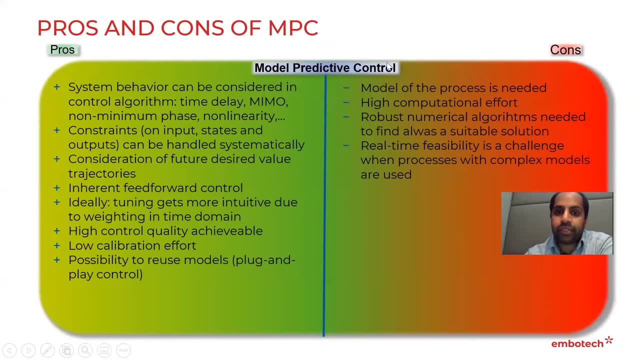 then we can still use everything else. so you see, there's a lot of advantages with model production control, but always when you have advantages, there's also some disadvantages. one disadvantage is you need to have the process model, and this needs to be a control oriented process model. so what i mean with it is if you have some models that are computation fluid, 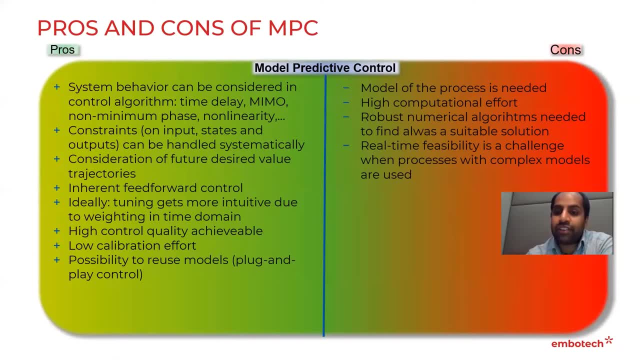 dynamics, where you have a lot of states and partial differential equations and very high complexity, then it's too complex to actually solve an optimization problem with it. so we need to boil it down so that it has limited complexity but it's still able to actually represent your input output behavior then, compared to classical algorithms like pid based control. 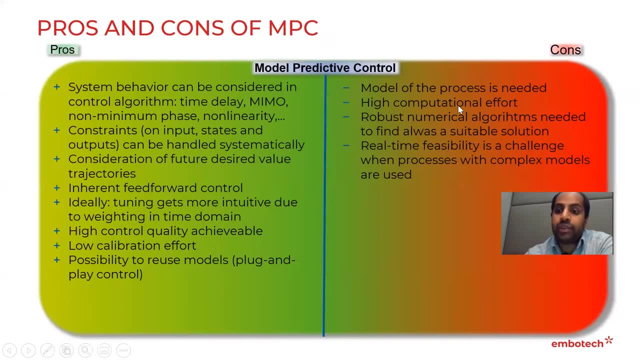 you have a higher computational effort, so it might be that you need to have a better hardware to actually run it on an embedded system. and the third point is you need to be very robust in terms of your numerical algorithms so that you find always a suitable solution. 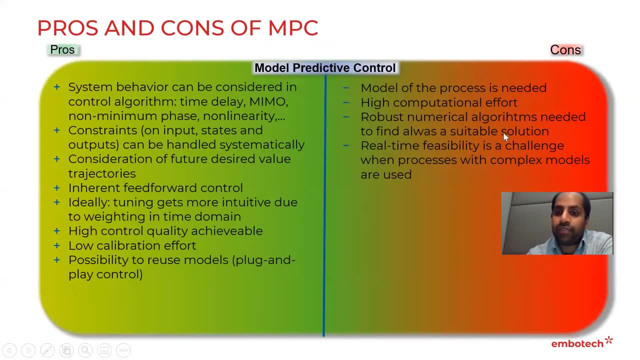 because with the prd based control, you know that you always have a suitable control action. and now that we deal with numerical algorithms, we also need to make sure that we always find a suitable solution of the optimization problem. and then, last point, this correlates to what we said before. so real-time feasibility is a challenge, and this is especially. 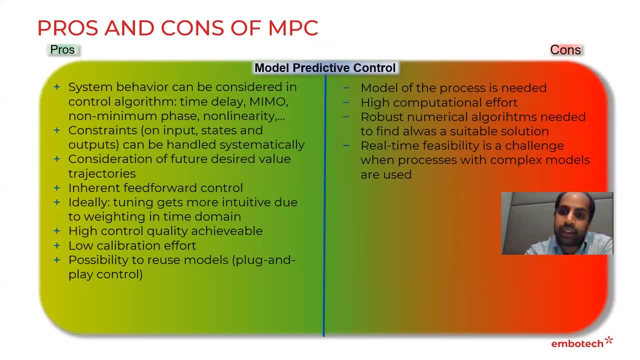 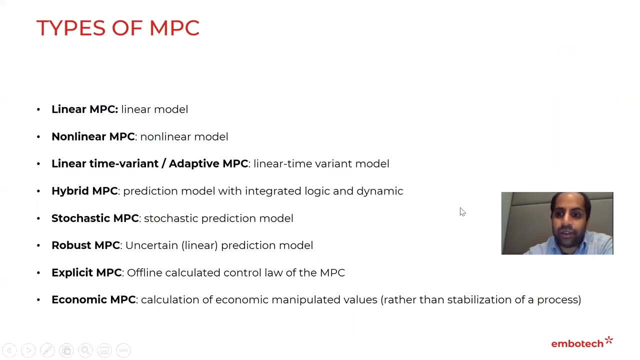 the case when we deal with complex models and, at the same time, have small sampling times, then you really need to make sure that, within the time frames that you have, that you are able to actually solve your optimization problem. good, so let's look at, uh, the types of mpc, because mpc- now i call that a control algorithm. 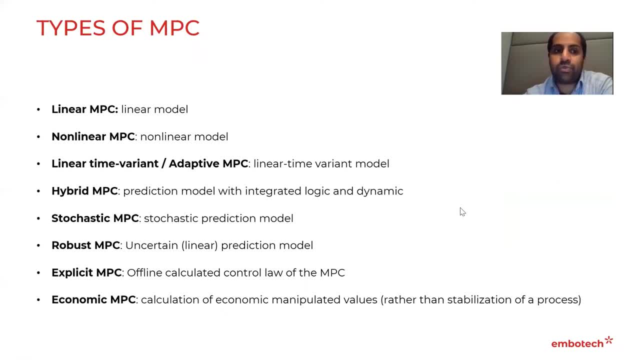 but actually, instead of actually being one control, i will. it's rather a family of algorithms and, depending on what kind of model you have, what kind of optimization problem you have, there's actually different names for it and different concepts also behind it, and here just the the most prominent ones which i put on the slide. 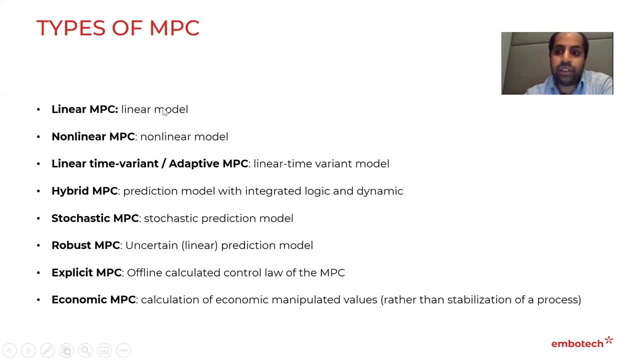 so if you have a linear model that you take into account for prediction and you have um also linear constraints, then it's typically called linear mpc. if you have now a non-linear model or maybe nonlinear constraints, then it's called non-linear mpc. one way in between linear, non-linear mpc is linear time variant or adaptive mpc. so some people 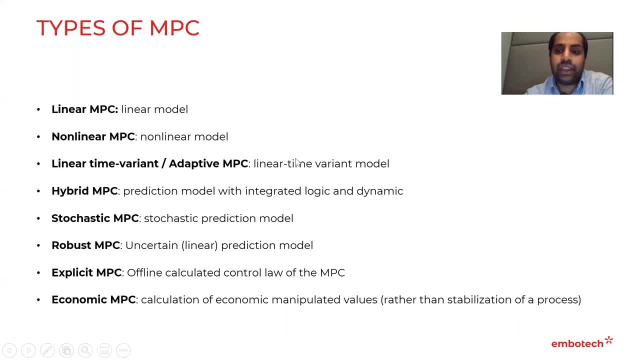 use the name linear timer and mc, others use the name adaptive mpc and there you have in every time step a linear model, but this model changes from time set to sign set. and then you could have hybrid mpc where you not have any more a continuous model, but you 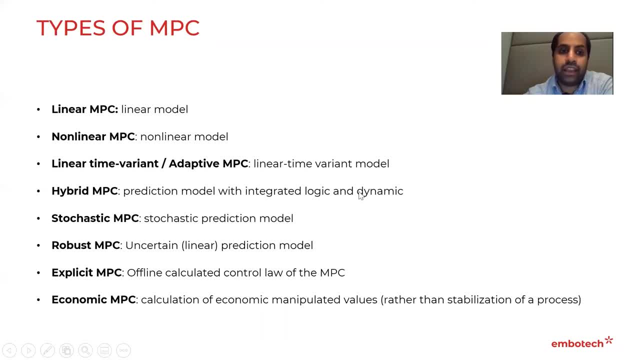 have a prediction model which has integrated logistics and dynamics and and then you need to solve mixed integer problems. then you might take into account stochastic information. so you have a stochastic prediction model. this is a. this is called stochastic MPC. If you have uncertainty in your prediction model, 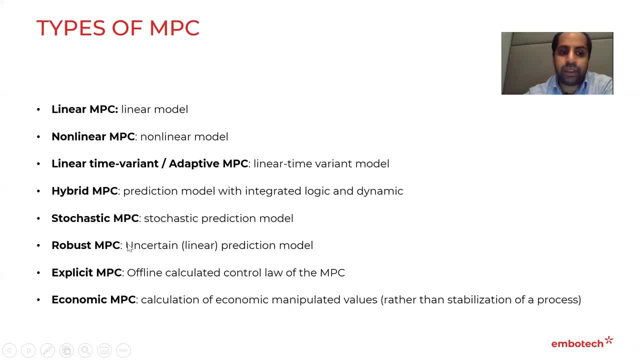 typically linear models are used, then you have a robust MPC, And what you can do as well is, instead of solving the optimization problem online during runtime of the process, you calculate your control law offline and you save just this control law, and then you just execute your control law online, and this is called explicit MPC. 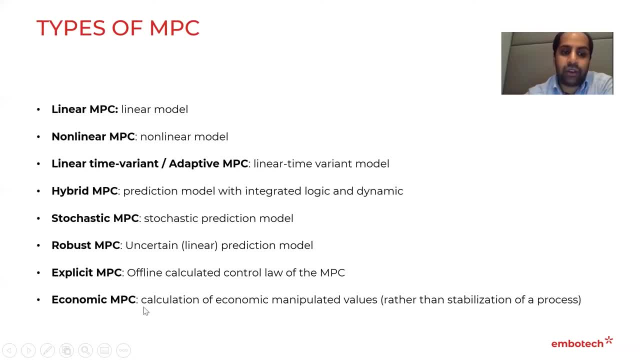 And the last one is called economic MPC, and there you calculate your economic manipulated values. So instead of having a stabilization process where you want to reference, track and have a stable system behavior, here the focus is rather that you have some control inputs that operate your process in a very economic way. 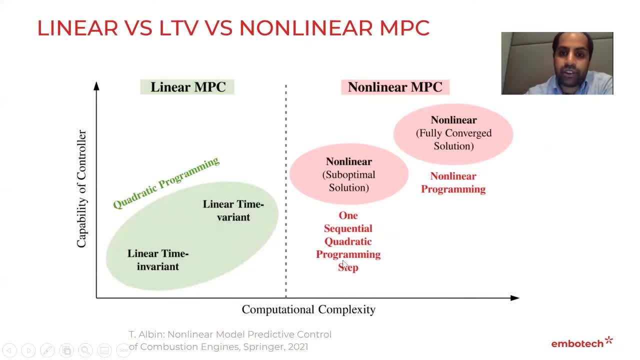 Good, and I just want to show you, like to give you an impression of the differences of the MPC and the MPC-MPC-MPC-MPC-MPC-MPC. So we have two axes: the computational complexity and what your control is actually capable of doing. 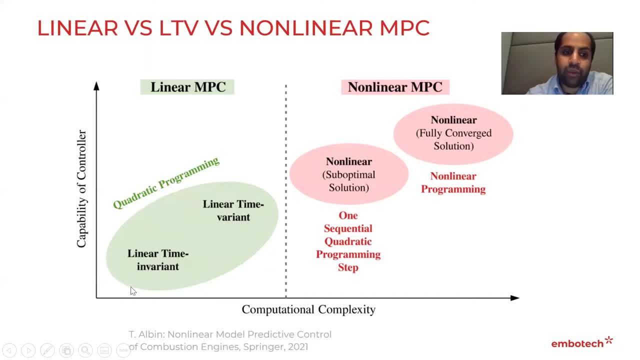 And if you have a linear time invariant model, then your computation complexity is very low, so you can solve it very fast. But on the other side, your control law will also only be able to handle linear systems or nonlinear systems that are not too. 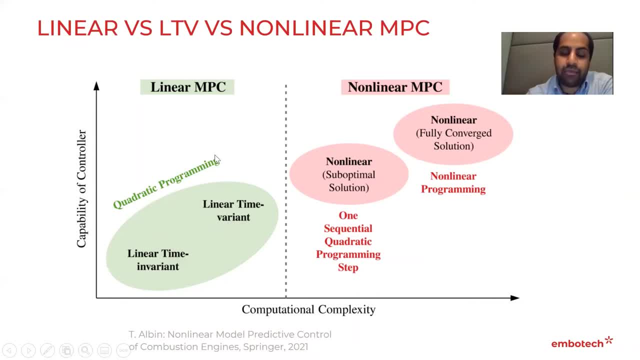 complex, And in this case you actually solve in each sampling step a quadratic program, and these can be solved quite reliably and also quite fast If you want to increase a little bit of complexity so that you are capable on the one side to control more complex systems, but with the 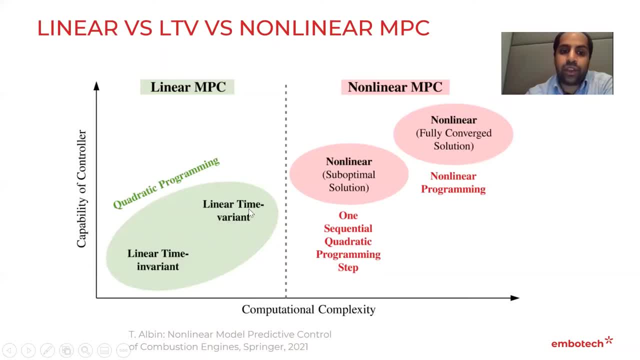 drawback of being computationally also more complex. then you can go to linear time variant or, as I said, also called adaptive MPC, And here you have in every time step a linear model, but it still resides in a quadratic program to be solved. 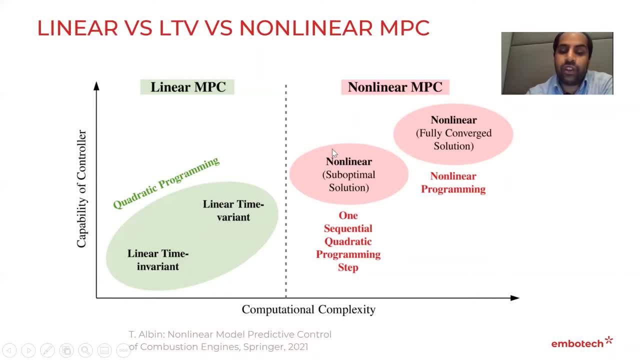 If we now go into nonlinear MPC, then you have a nonlinear system model that you are looking at And in this case you solve actually nonlinear programs. and there's two ways to deal with it. And you can either, in each sampling step, just calculate a suboptimal. 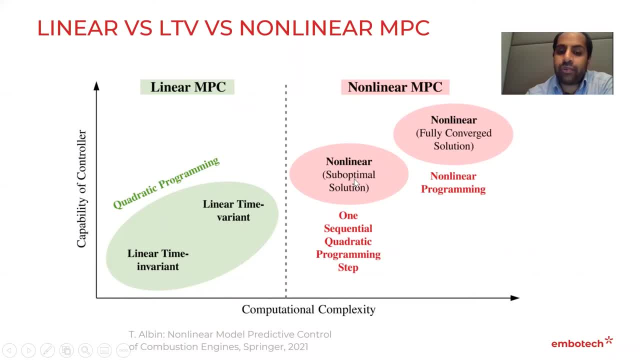 solution, So you don't converge your optimization algorithm to the end, And one method that is often used is that you solve only one sequential quadratic programming step, and this is often called real-time iteration scheme, And in this case you have a little bit. 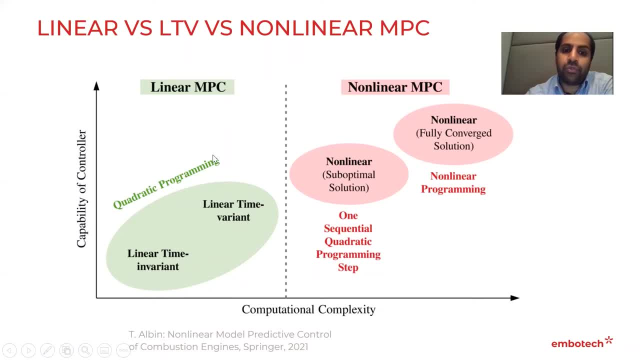 higher computational complexity, but you can already control more complex systems And often this nonlinear, suboptimal solution you can use. actually, if you have reference tracking problems- Yannick Mahéle- And for For these they are quite suitable actually. 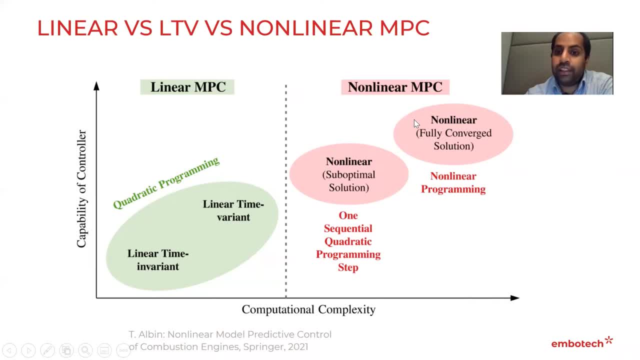 And the other case is that you have a nonlinear system model and you converge in every iteration step to the fully converged solution. And this is often the case in motion planning problems where the suboptimal solution is not enough but you really need to converge. 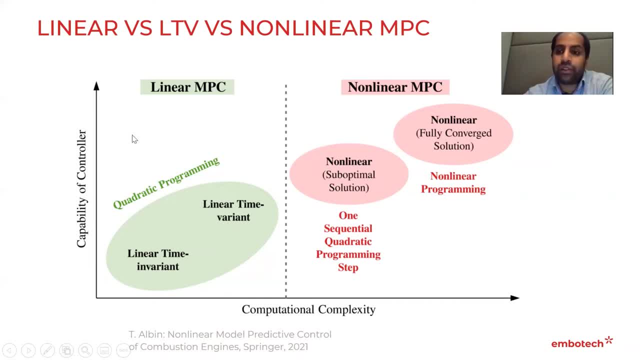 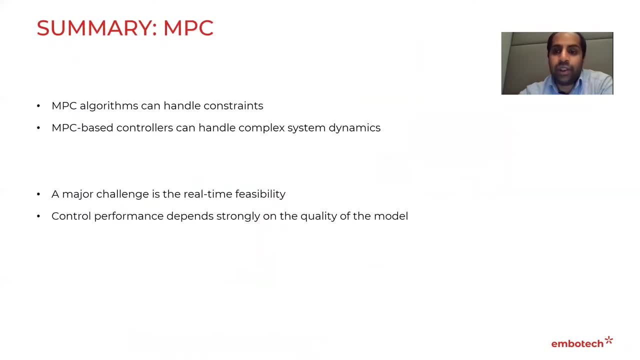 And then you have the highest computational complexity, but then your controller is also capable of doing or dealing with very complex systems. So let me give you a summary. So MPC-based algorithms: they are superior in terms of the control quality. You can handle constraints in a systematic way and you can handle very complex system. 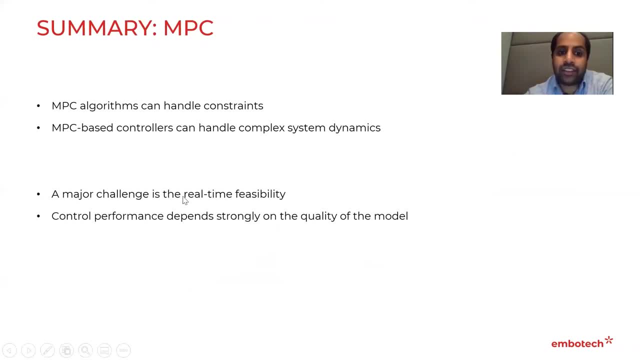 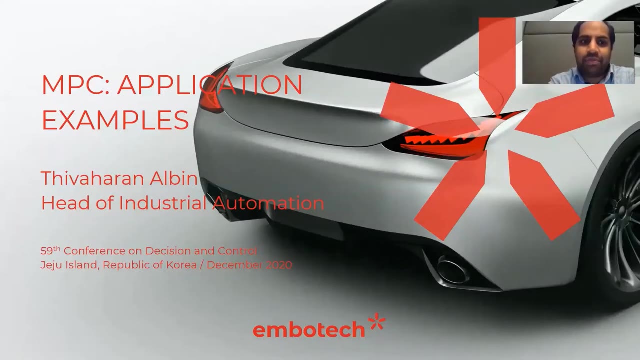 dynamics, But on the other side, a major challenge is the real-time feasibility, and your control performance depends strongly on the quality of the model. All right, Let's now look into some application examples where actually model predictive control is applied, And for that let's start with a little bit of history of MPC. 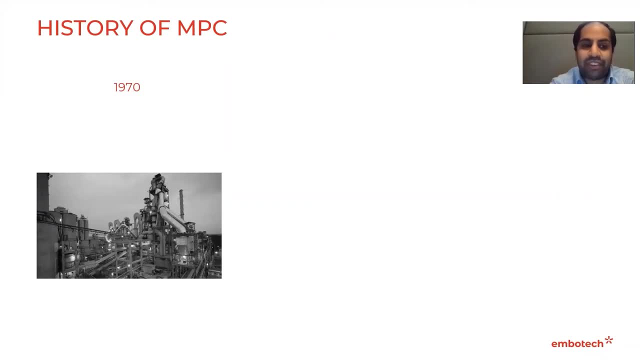 So going a little back in time, so around 1970, actually MPC evolved in the process industry. So, for example, you had chemical plants which were controlled by model predictive control And it was a great success story there And it got implemented in more and more applications in the process industry. 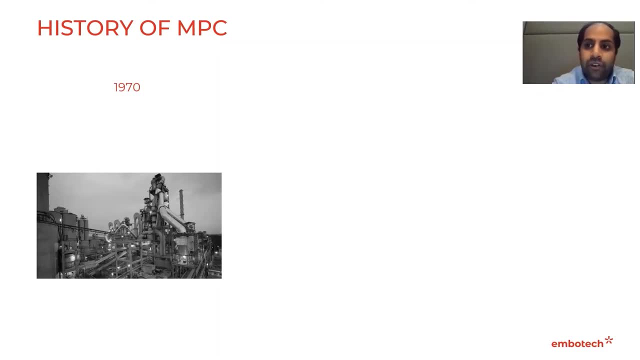 And these were actually applications that were characterized by rather long sampling times and small or slow dynamics. And the nice thing is, in the process industry you can have still some quite powerful computing units to actually calculate that. So let's start with the MPC. 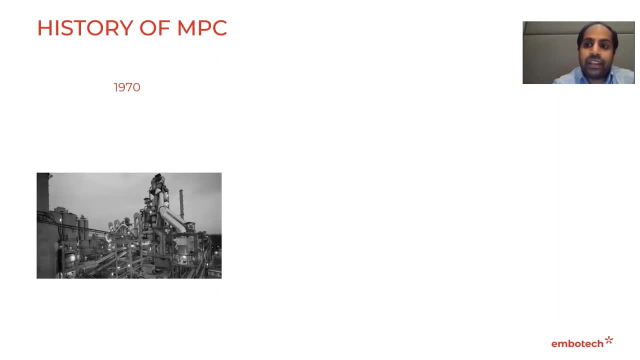 So the MPC actually has a lot of interactive values. So it was quite nice environment to actually apply MPC And so you had a lot of gain, because if you are able to increase the productivity in such a chemical plant, then of course you have a list of money that you actually would save. 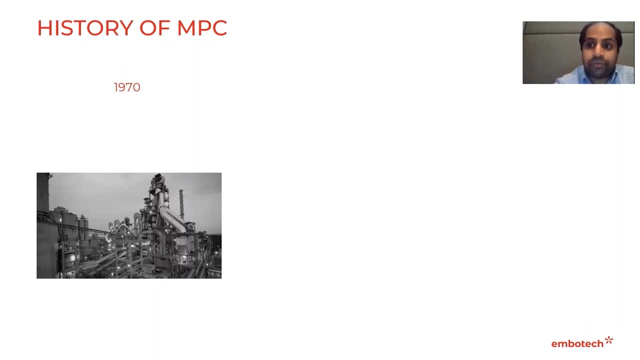 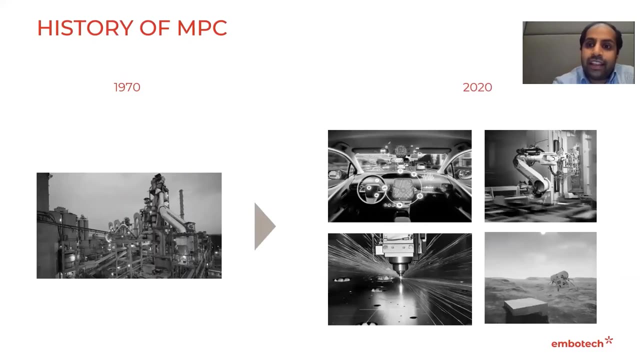 because you're operating the process, for example, more efficiently. If you now look into examples of applications from today, then these are actually fields like autonomous driving driving, robotic motion planning, CNC machines or guidance and control for aerospace systems, And what are characteristic of these examples are actually that the sampling times are very 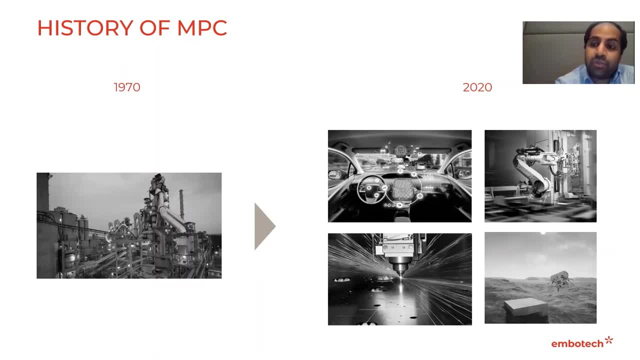 fast, so very small sampling times, so you need to compute very fast. At the same time, it's often embedded systems, so you're not able or you need to be capable of solving the whole problem with this limited hardware that you actually have. 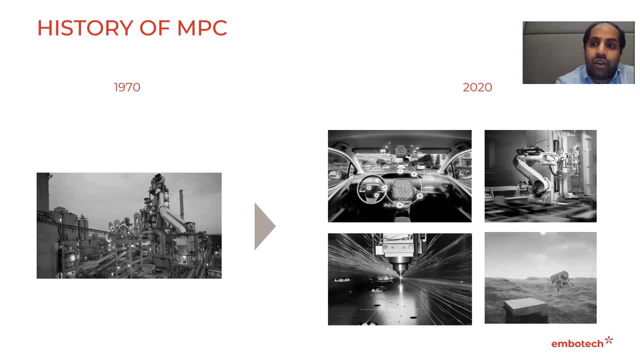 And one other big distinction from the early developments of MVCs in the process industry: you still have an operator who's sitting there and you exactly know what is happening. What I mean with that is you have a set point which you need to follow, but you know exactly. 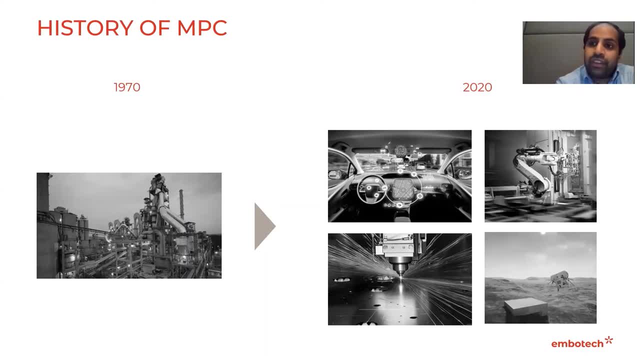 what the set point curve looks like. If you take autonomous driving, you don't know in advance what actually the driver will be doing, so you need to be capable of handling any reference change that is actually upcoming, So meaning that the applications that are at the moment evolving or where it is actually 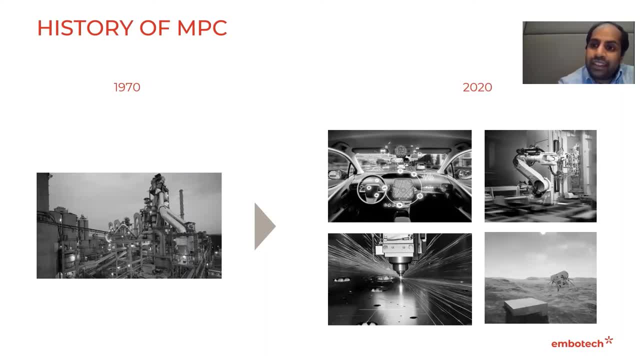 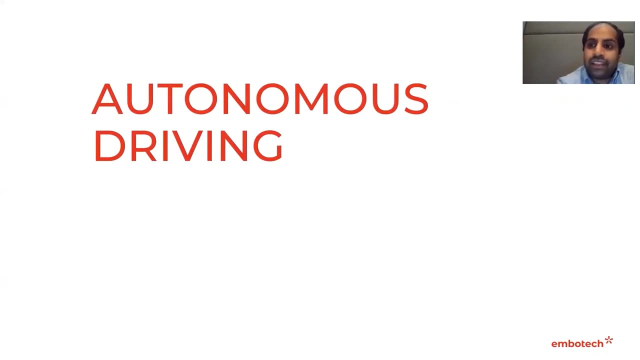 applied. they are characterized by the need of very high reliability and the limited hardware where you need to compute everything on. Let's look a little more in detail. I'm going to start with autonomous driving and then on the other side into smart factories. 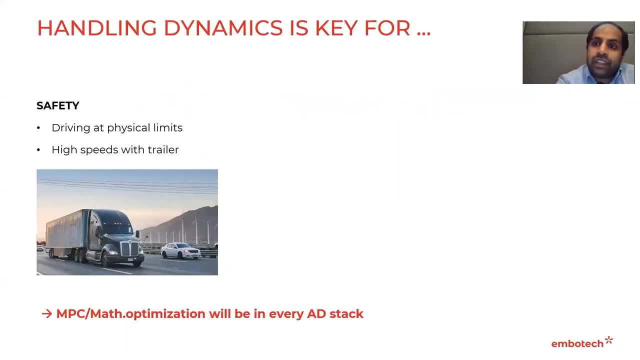 Starting with autonomous driving, one key point for autonomous driving is actually being able to handle the vehicle dynamics, And you need to be able to handle the vehicle dynamics due to different reasons. The first one is safety, so you need to be capable of driving the vehicle at the physical 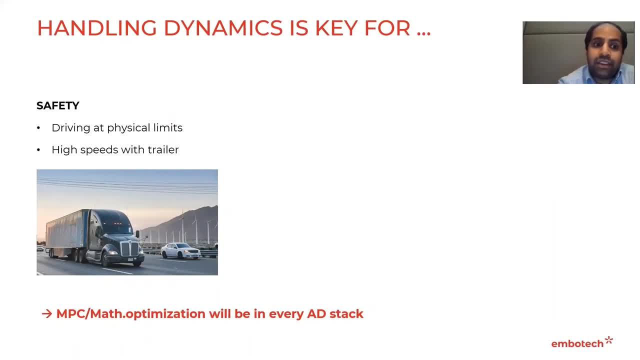 limits. So you always want to have a stable behavior so that you're safe. And this is even more complicated when you have a setting, as you see here in the picture, where we have a truck, where you drive high speeds with a trailer and then the vehicle. 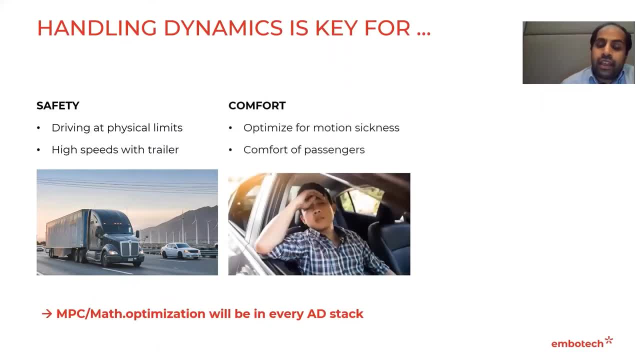 dynamics gets even more complicated. At the same time, you want to be, you want to drive very comfortable, So assume you are oscillating around, But then you would actually get motion sick. That's what you not want. Instead, you want to have or offer the passenger a comfortable ride. 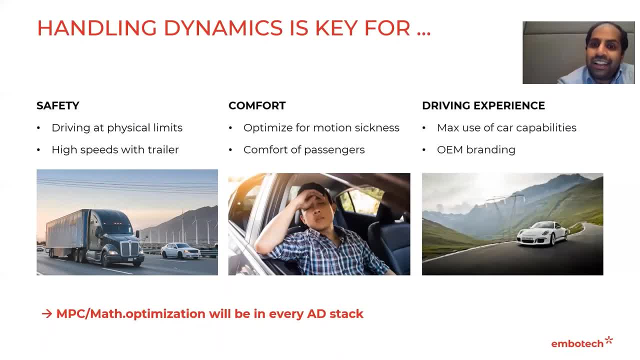 Then the third point is you also want to give the driver a certain driving experience. So let's assume you have a sports car, then you want to use also what you have in terms of car capabilities. And you see, like these requirements, these different aspects, let's call them and they 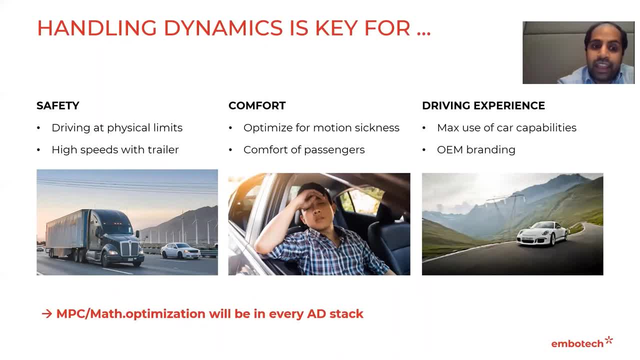 are quite complicated. They are complicated to satisfy at the same time- And here, in this case, MPC and mathematical optimization becomes very crucial because you are able to actually fulfill all these requirements. And MPC, mathematical optimization, will be in every autonomous driving stack because 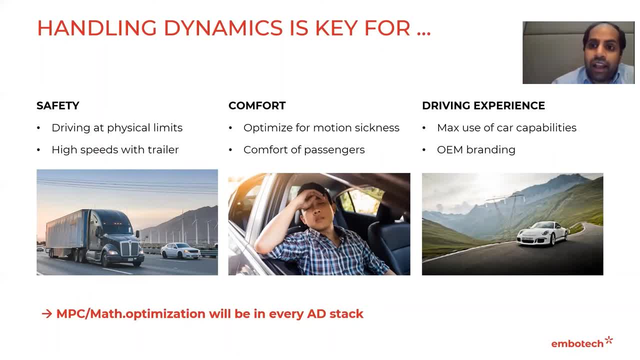 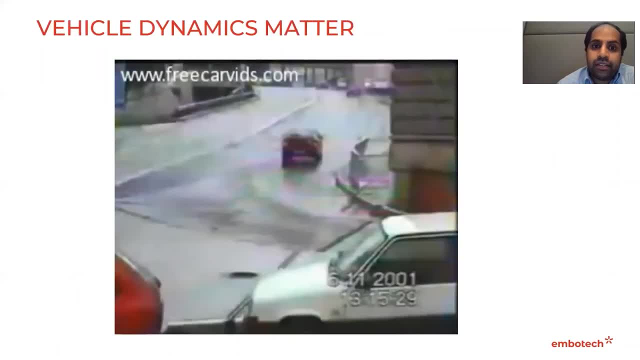 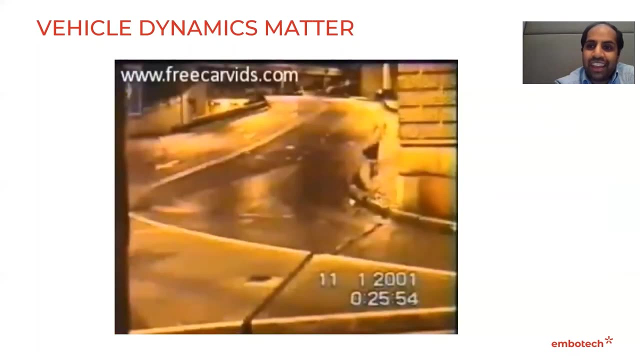 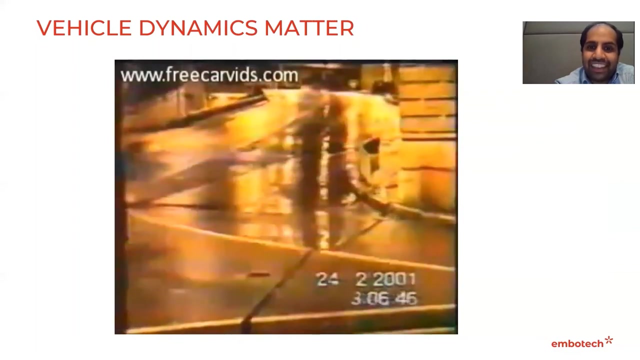 with classical controllers, it's very, very hard to comply with all the different aspects. So now you might say, Well, let's look at the vehicle dynamics, that can't be so complicated to be able to deal with it. But now let's look at this video where we see actually how complicated it can be. 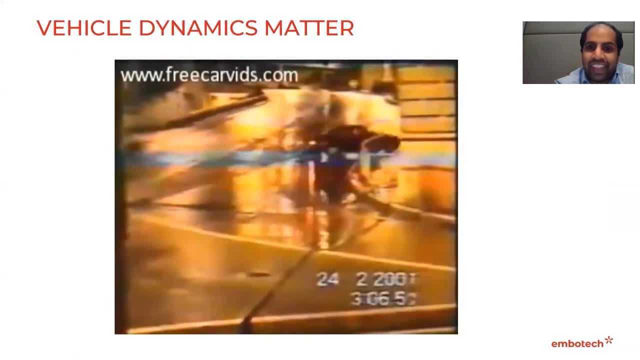 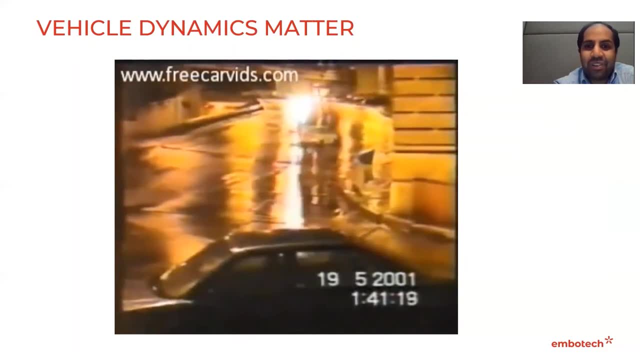 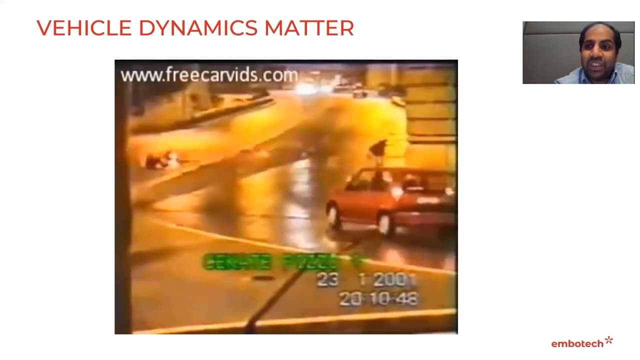 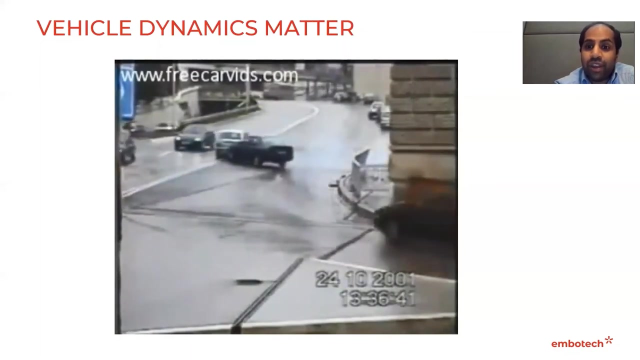 So you see the cars that are sliding around the corner, And so, it seems, the human driver is not always the best at knowing the physics and knowing the limits of the car. And, of course, if you have an autonomous driving car, Then you want that the algorithm knows this physical limits and is capable of still driving. 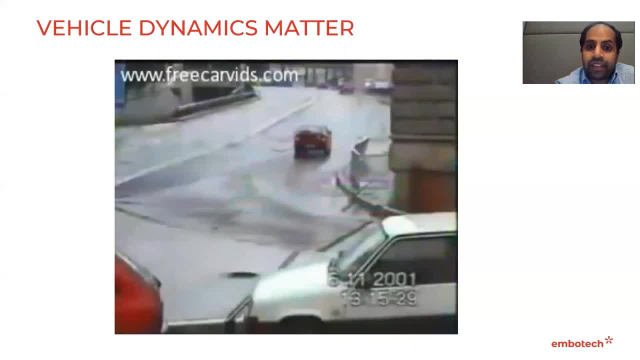 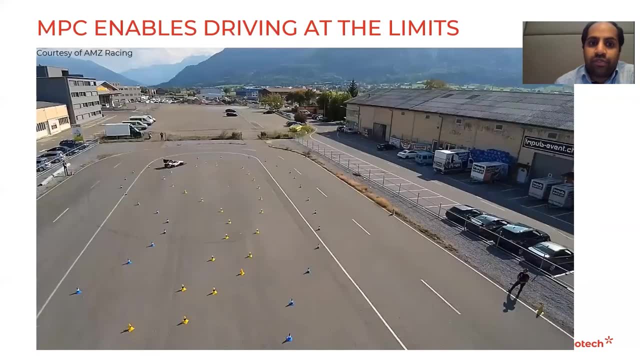 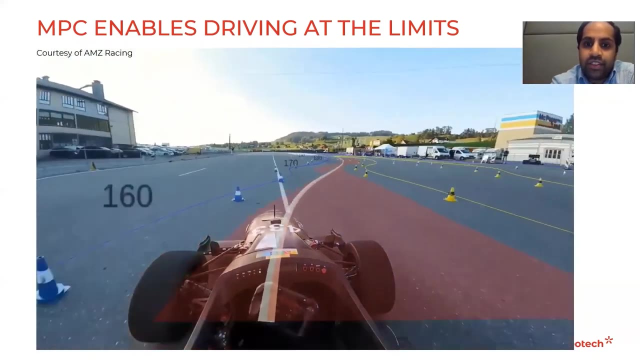 safe even in these scenarios. I will show you that MPC is capable of doing that with three different scenarios. Let's look at the first one, And this is done by AMZ Racing, which is an ETH Zurich student club for racing, And they use actually forces based. 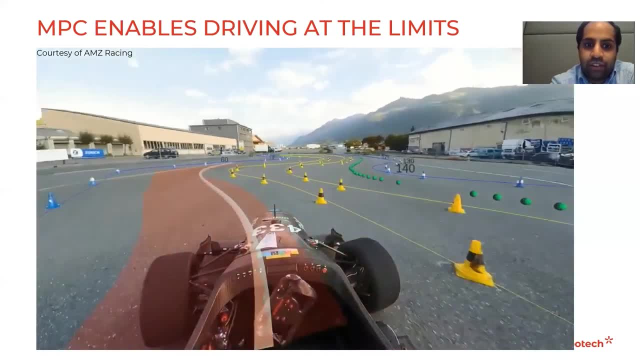 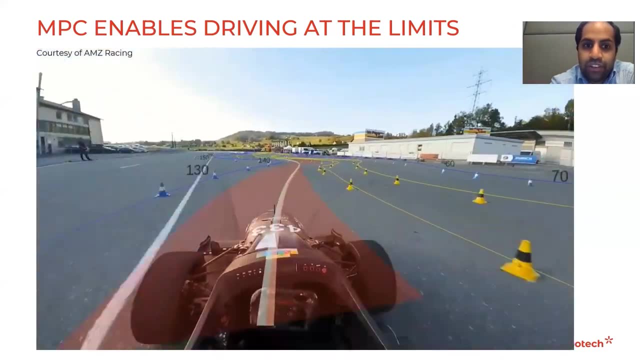 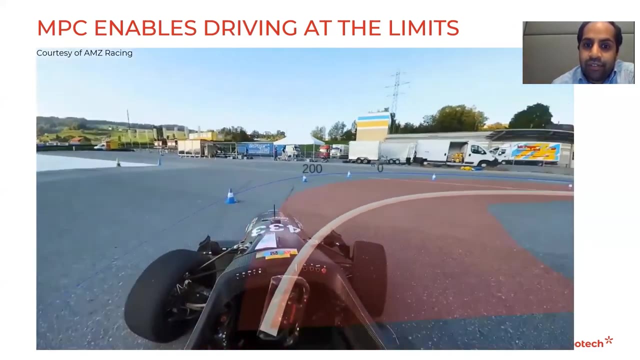 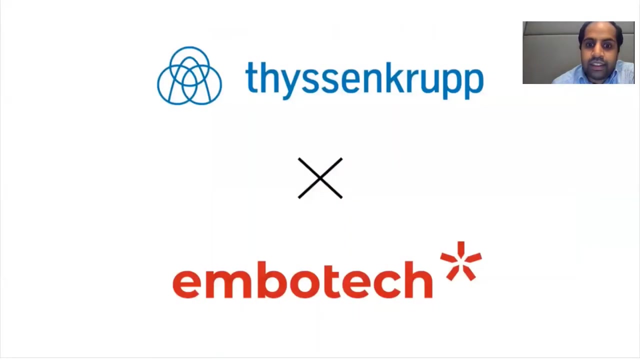 Motion planning algorithm to drive an electric car- And they actually have won a competition with that- And they're able to steer around this at the various corners and handling the dynamics in a very nice way, so that you're still able to have a top performance. 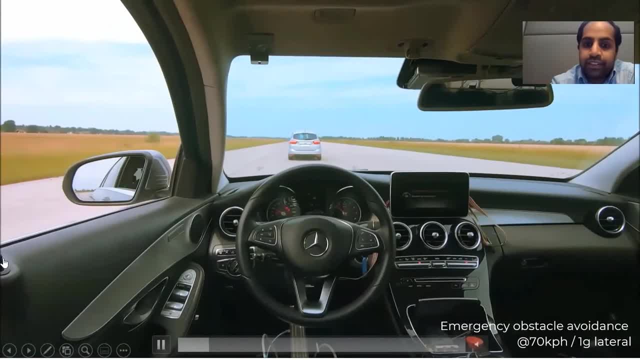 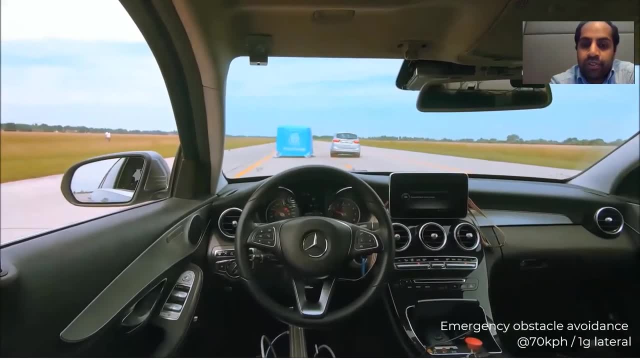 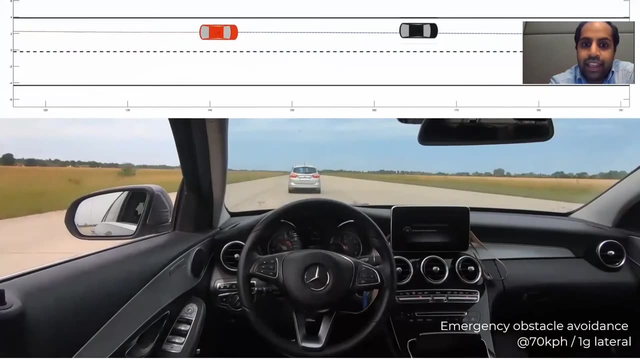 The second scenario I want to show. It's also forces based Motion planning algorithm And there we have a commercial vehicle And it's also driving autonomously And in this case there's an obstacle place And you only see in the last minute actually that there is an obstacle. 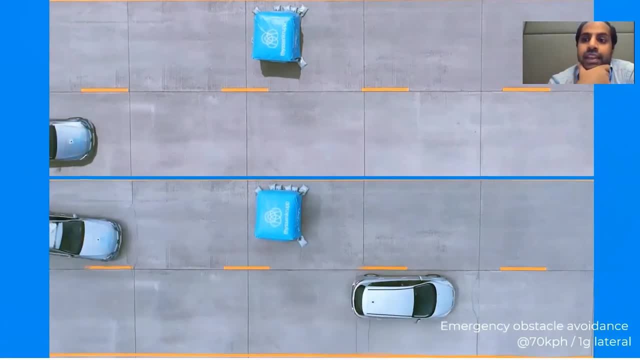 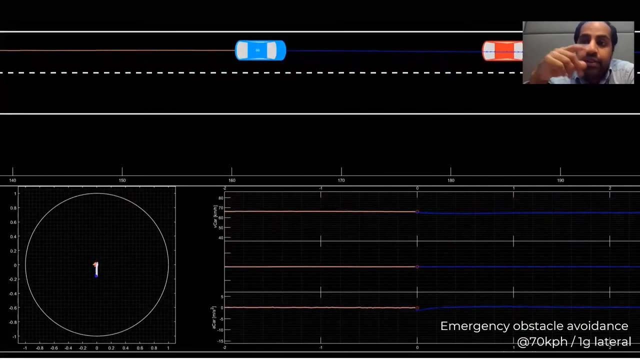 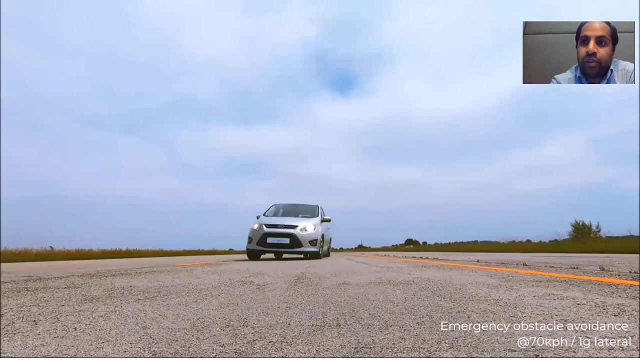 And due to the update rates of the MPC algorithm. Actually, the MPC algorithm can actually calculate an evasion maneuver And you just saw Like if you would just brake, you would actually run into this obstacle. So the only way to be safe is actually to avoid it. 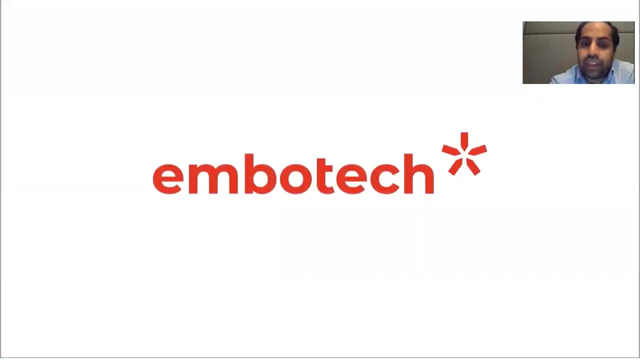 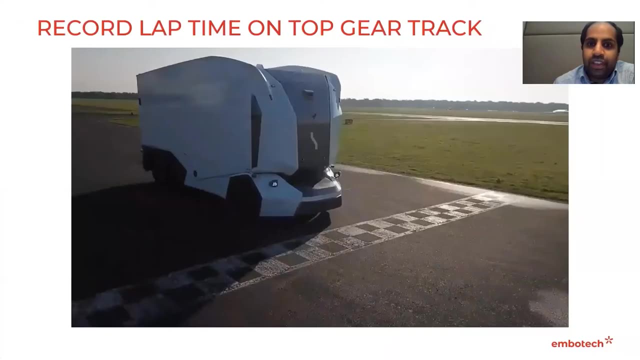 And this can be done in this way, And this was a cooperation of Emotech and ThyssenKrupp. As last scenario, I show you a motion planning algorithm which was also developed forces based together with Einride, which is a Swedish startup. 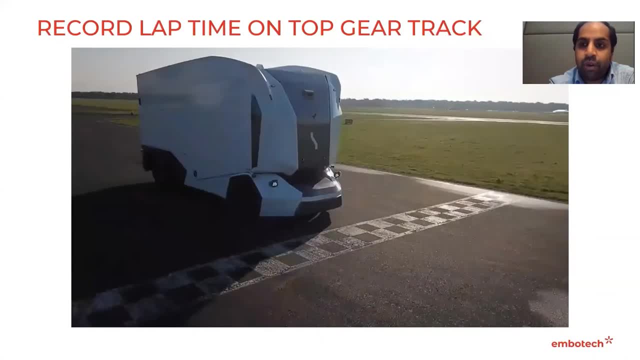 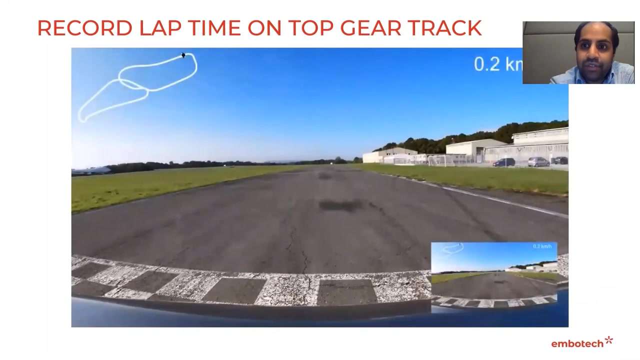 That actually builds electric pods that actually are able to autonomously deliver goods. And here you see the top gear tracks from a British TV show And they are actually also autonomous. The pod is driving autonomously And with the motion planning capabilities the MPC based, it was actually able to set. 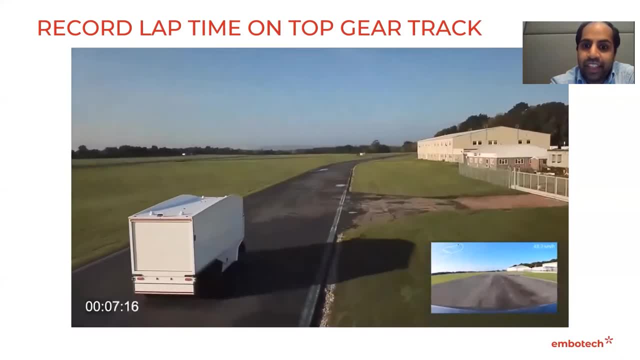 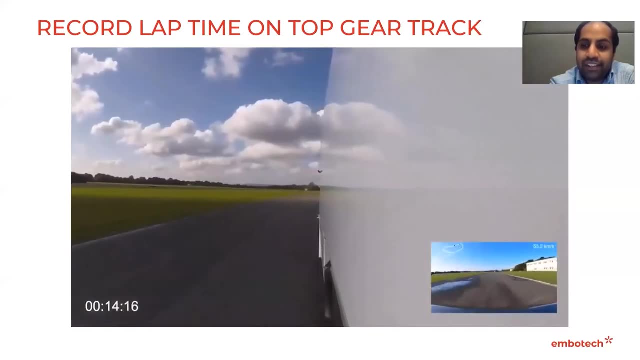 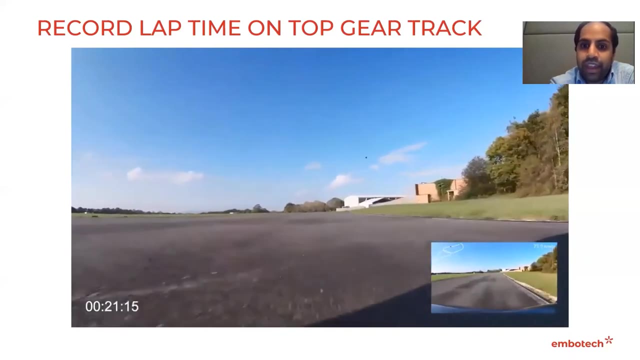 a record lap time on this top gear track And here again, different vehicle configuration, but still you are able to take the dynamics of this vehicle into account And then you are able to actually drive optimally around the lap track. to be as this was the 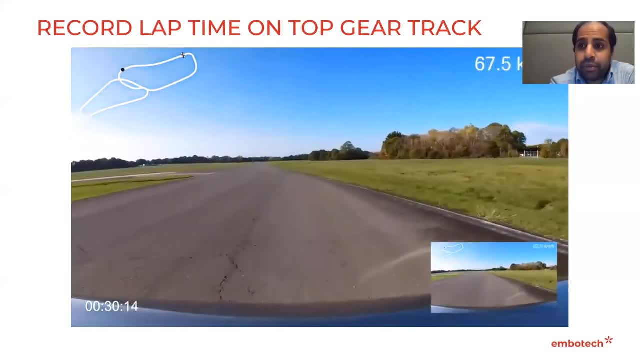 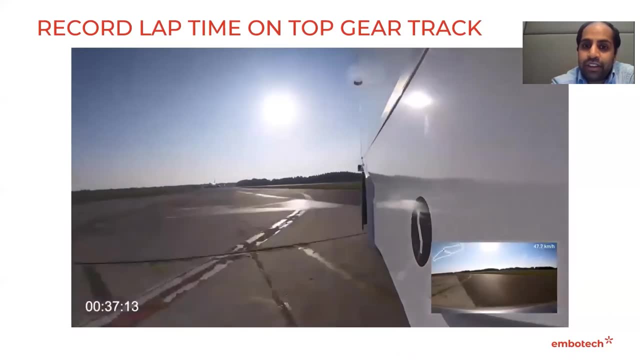 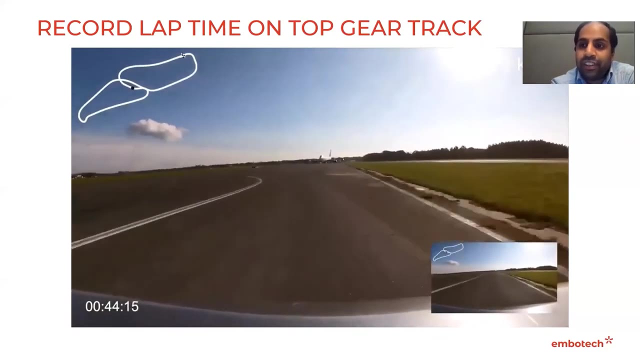 goal here to be minimal in time. But the beauty, of course, of MPC is to see It doesn't matter if we have the electric driving racing car or the standard vehicle or this pod. here You can actually model the vehicle dynamics of these systems and then plug it into your 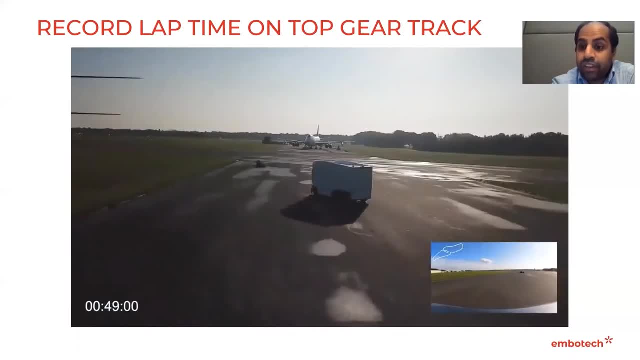 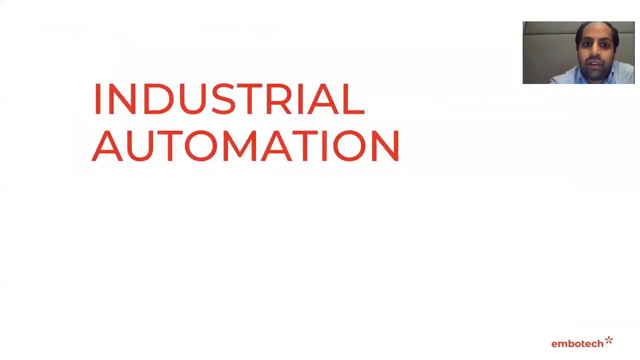 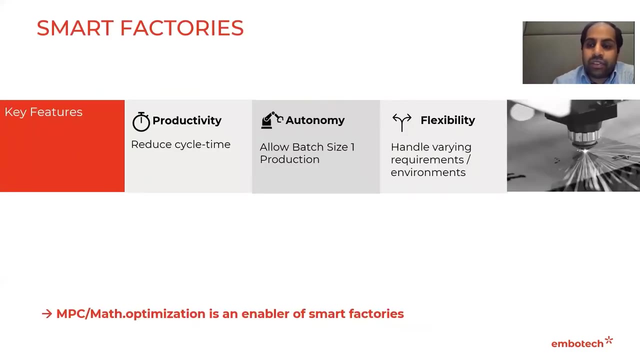 algorithm, And then you are capable of actually solving this motion planning problems. Now let's look into industrial automation- And we are going to talk a little bit about industrial automation- And where MPC can be applied there- And let's look specifically into smart factories that are more and more evolving. 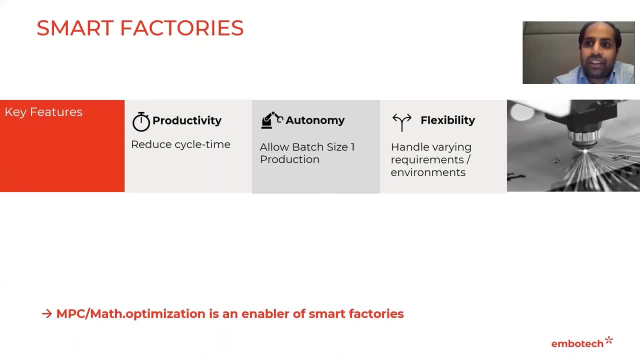 And if you have these smart factories, what you actually want to do, what is your goal at the end as a manufacturer? you want to be as productive as possible, So you want to produce as many goods in the lowest time, So you want to reduce the cycle time. 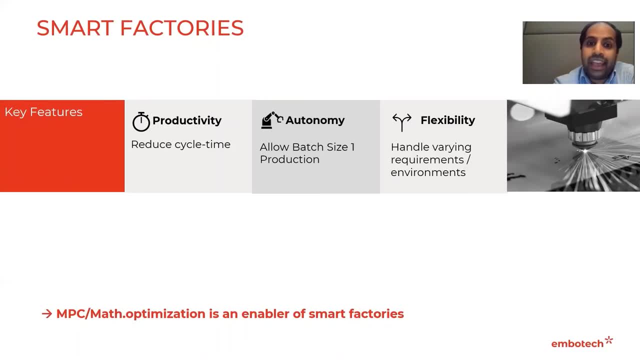 Cycle time is the time that you need to produce a good And, at the same time, as the products get more and more complicated, More and more complex, And you get more and more variants of products, You want actually to be able to have a batch size one production. 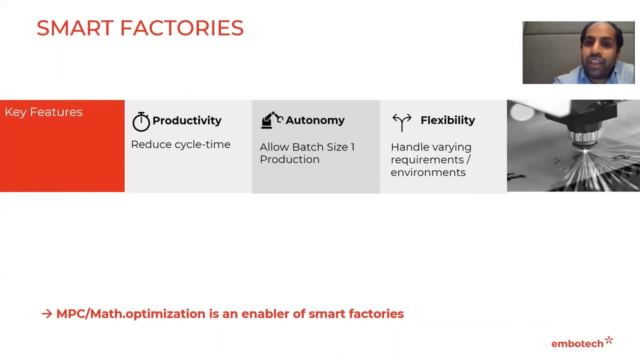 So it means, even if you change all the time your product that you produce, you want to be good. So what you don't want to do is that you have a lot of change time and then you need to set everything up again and then you produce a new part. but you want to get it down that 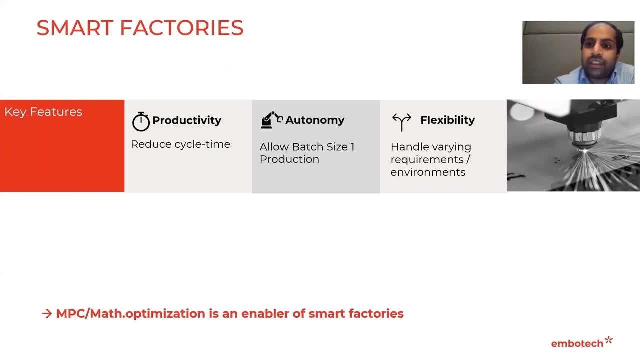 you have an autonomous production systems and it doesn't matter how big the batch size actually is, You still are very productive. The last part is you want to be very flexible. So even if you have varying requirements, because you have different products that all have- 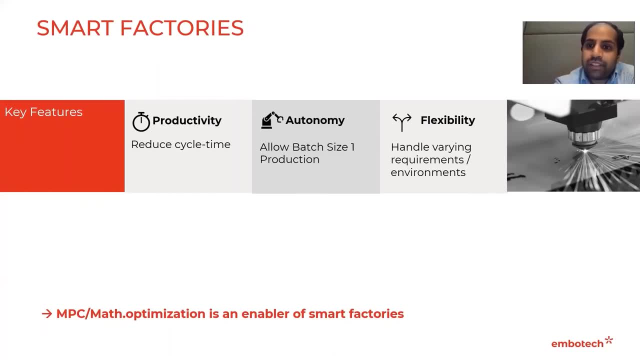 specific needs or you're changing your environments, that you're actually capable of dealing with this. And here again, the MPC and mathematical optimization is actually an enabler for these kinds of smart factories, And I want to show here again some scenarios. So the first one is also a 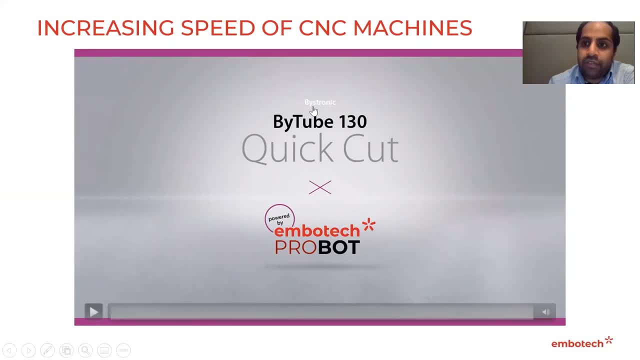 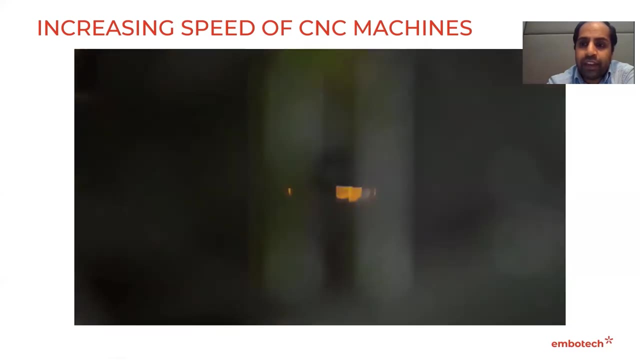 A forces based solution which we developed together with Bistronic, which is a laser cutting company company from Switzerland, And here we use it actually to control CNC machines And in this case there is a redundant axis. So you have one movement which you can actually do with two different axis and the two different 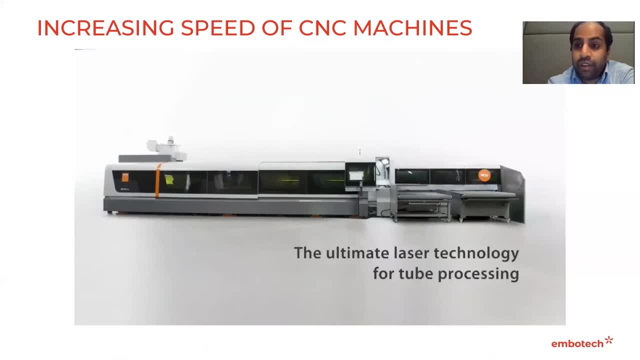 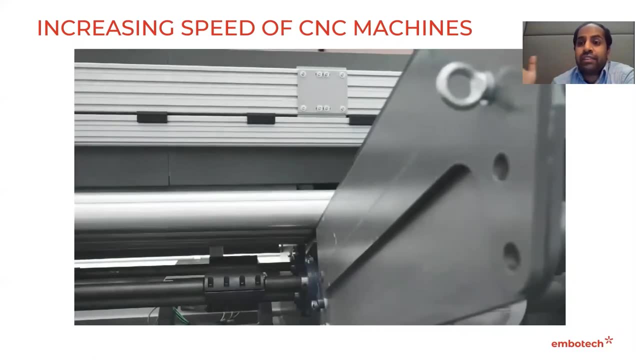 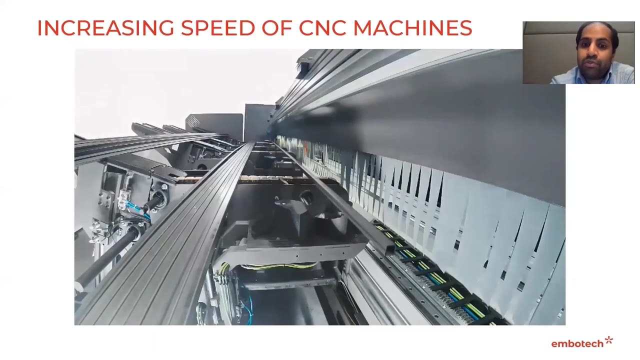 axis. they have different characteristics. The one is very fast, But You can only move it a certain distance. in the other one, You can move over a long distance, but this is a little bit slower. And now the question is how to optimally split the movement along these two axis. as to that, 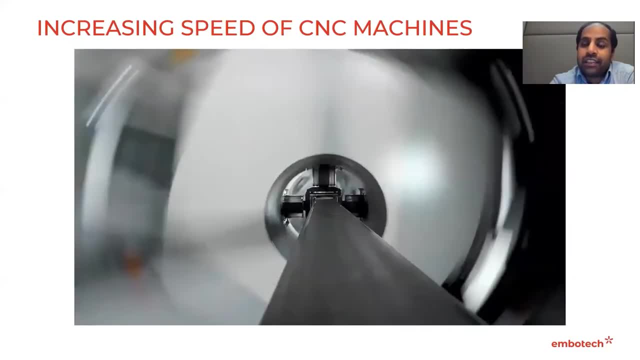 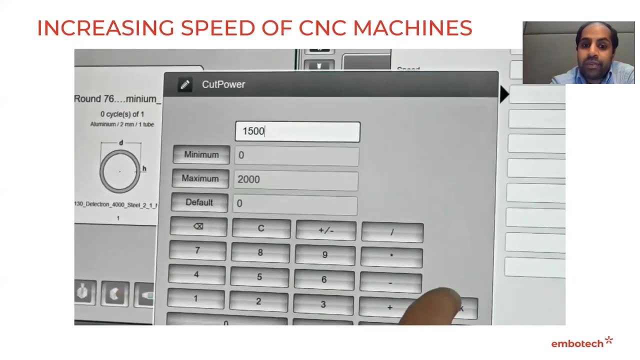 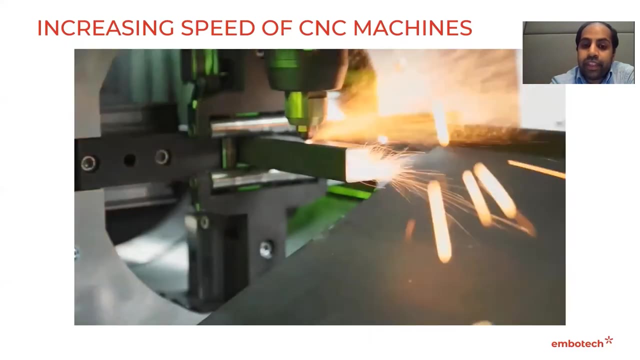 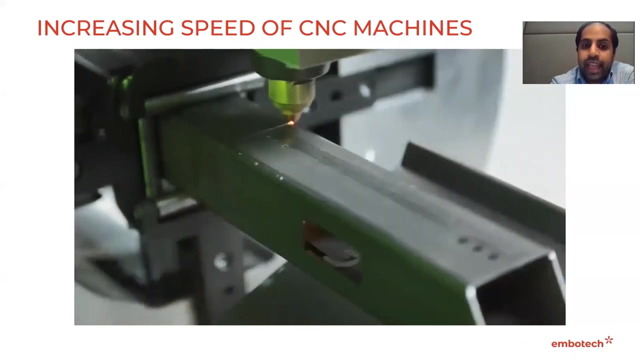 you are on the one side, that you are really fast, But of course, as it is about cutting, you need to be, at the same time, very precise, And this is what we did, also with an MPC based solution using forces, And there we were also able to increase productivity by up to 10 percent. 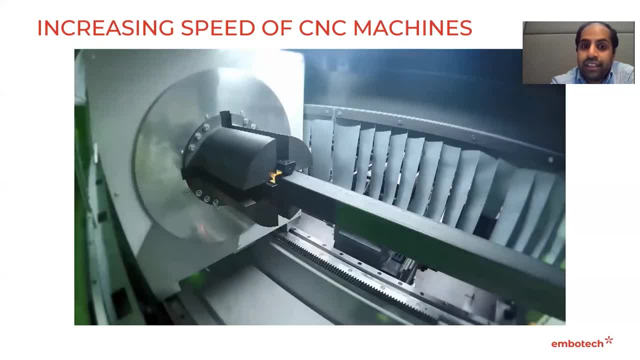 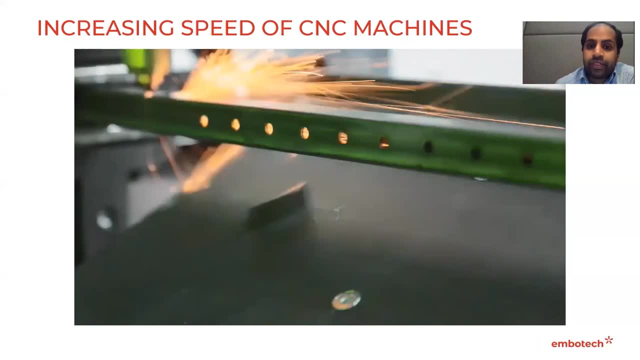 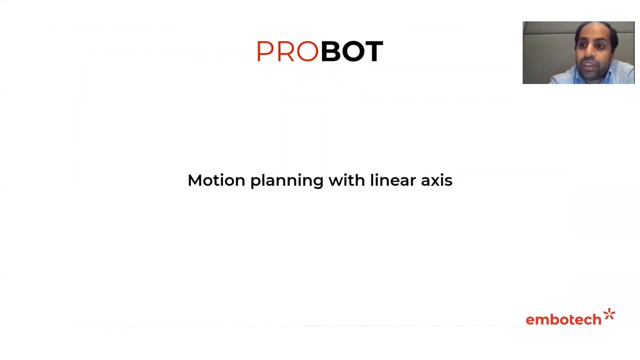 And this allowed the laser cutting company to actually deliver a solution which is much faster as what their competitors actually have. Another very interesting topic is robotic motion planning. Also here again, as I said, It gets more and more flexible and you want to be able to do the robotic motions more. 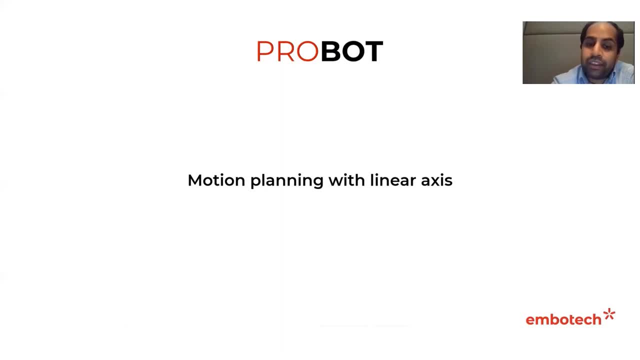 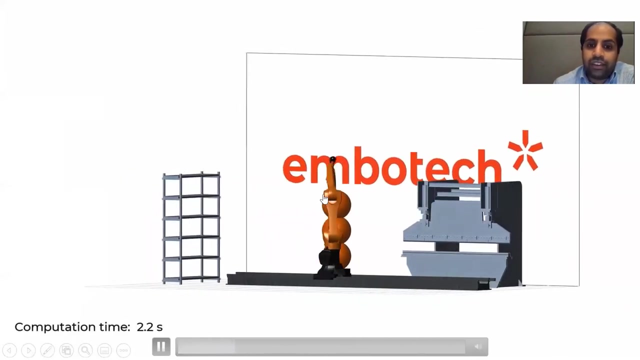 and more non static and in a more dynamic way, And let's look into one example, which is motion planning with a linear axis. So what we see here is we have a manufacturing process and you have a shelf with something that you pick out and on the way you have some obstacles, and just for demonstration. 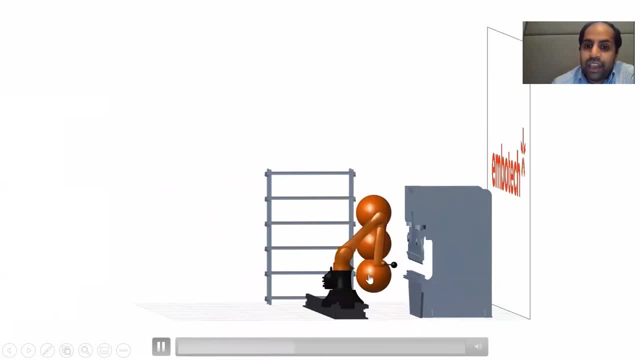 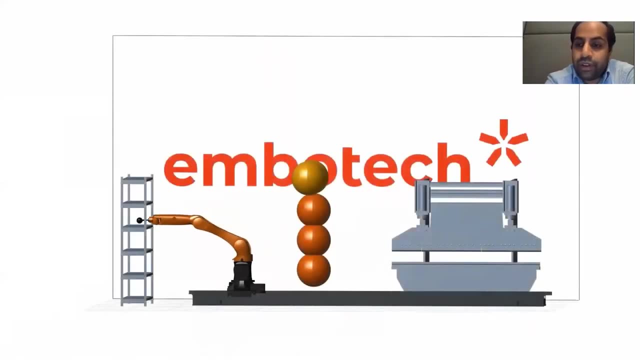 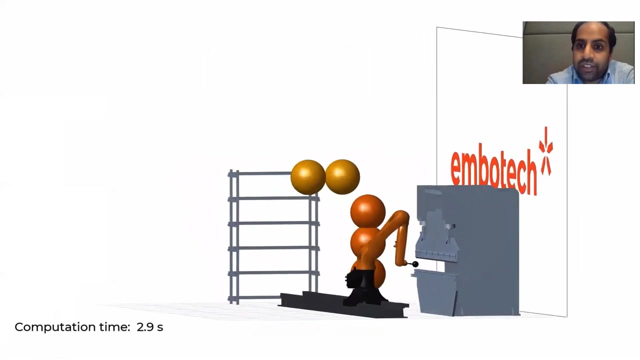 purposes. These are now some spherical obstacles, And what you want to do is actually, if the environment changes because the cell has a new structure, that you actually update your motion plan and that you can continuously run this operation even though the cell is changing. 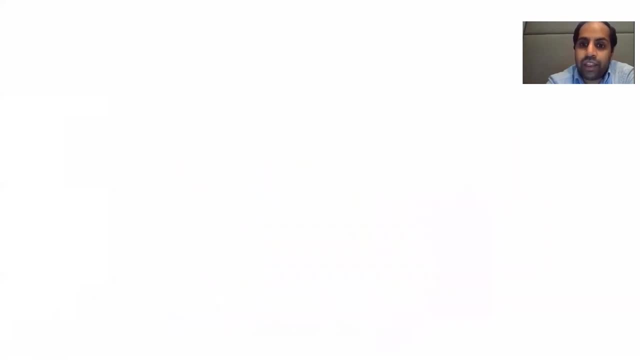 And you saw, in this case you are in a few seconds, you are able to actually recalculate the best path to get time of the really from the shelf to the manufacturing Place. And another example that gets even more complicated is if you have two robots that work together. 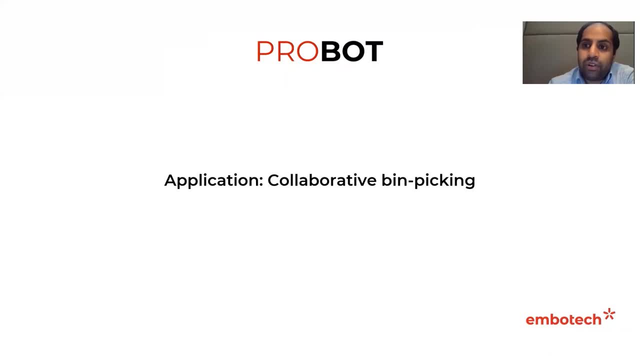 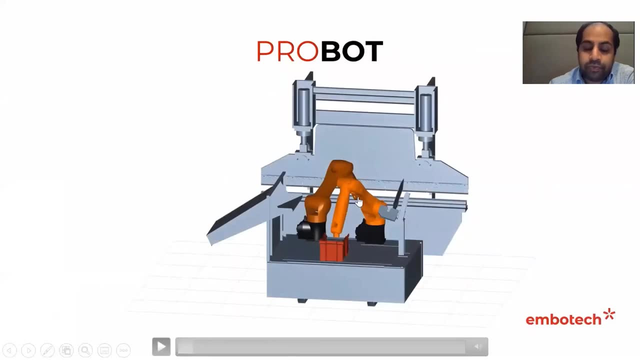 in one cell, And so this is collaborative bin picking. So let's look at this. So you have two robots here And, as I said, you want to increase the productivity and reduce the cycle time. and the main bottleneck here, This cell is the. 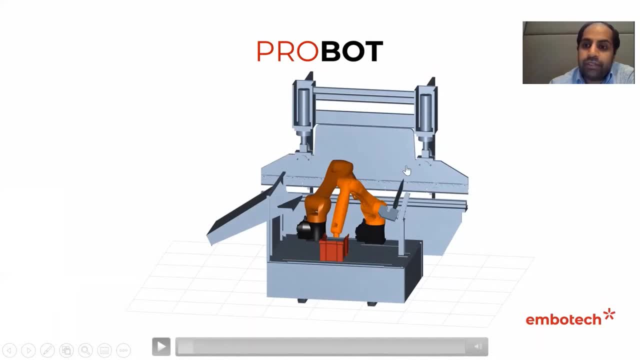 The manufacturing place here in the background And you want to use that as much as possible. and what it's done to actually realize it is. you have two robots that work synchronously and you need to plan the motion so that they optimally do their tasks. 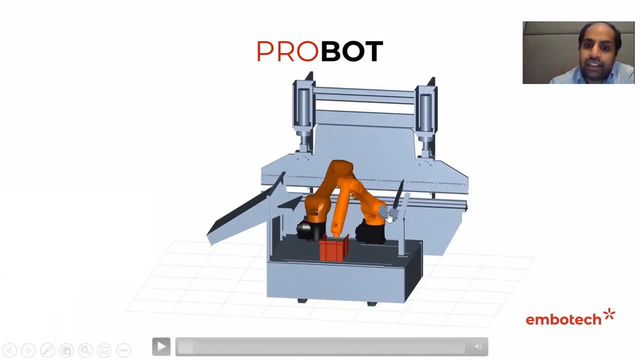 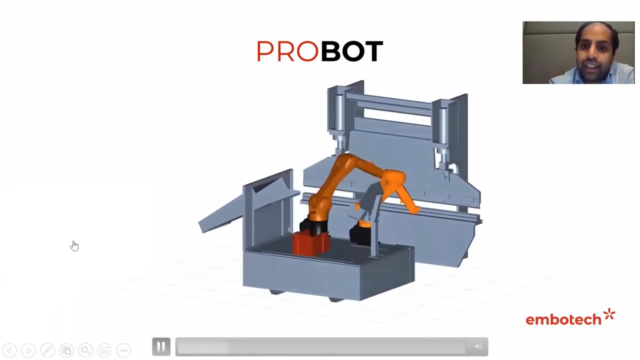 And what they do is they pick out of the bin a metal sheet and they do some alignment on this alignment station, Then they do the manufacturing process and the manufactured part then gets deposited into this bin. And you see, now the motions of the two robots are calculated such that they are optimal. 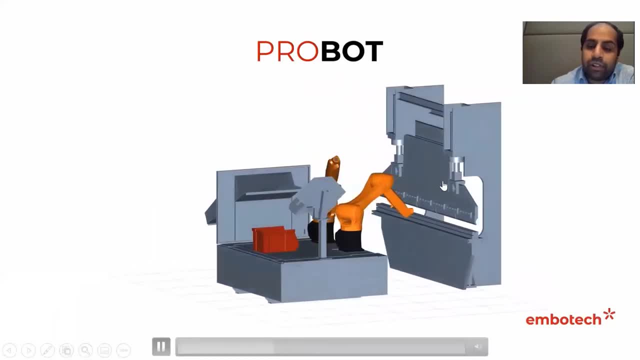 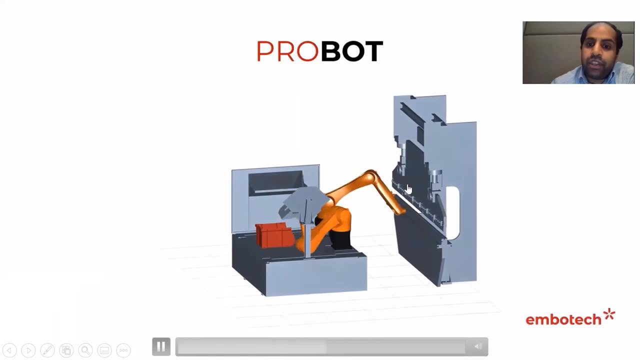 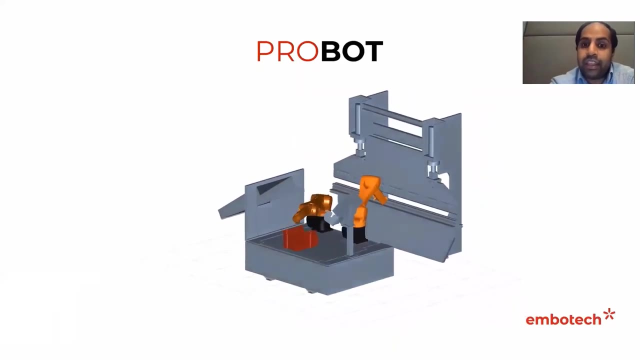 And then, as a result, we can use as much as possible the manufacturing place here, And if you would only have one robot, you would spend quite some time to go around, but not actually with manufacturing the path, And for this, of course, this is MPC also again, but you need to take into account both. 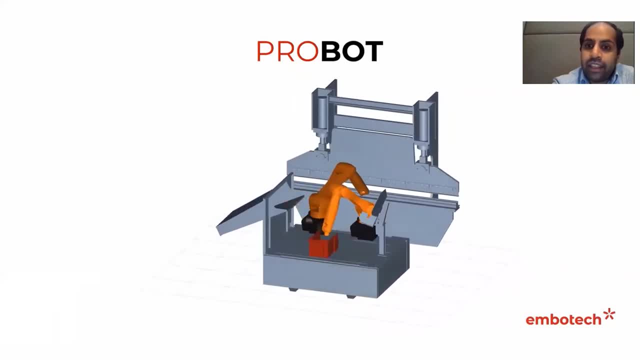 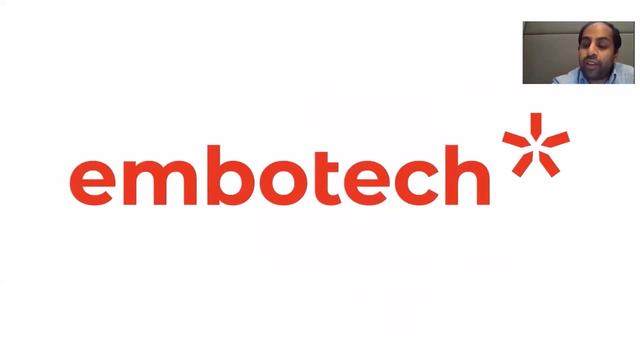 robots, So that you have a motion plan that takes into account what the other robot is specifically doing and that you have a joint movement that is optimal in time but where you don't collide into each other. All right, I hope I could give you a little bit of an impression of what current topics